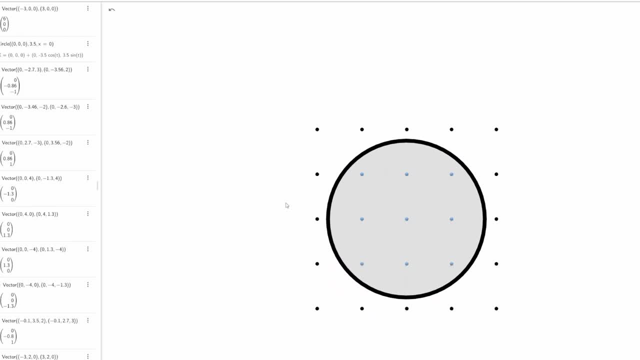 tell which ones they are. Looks like that. So a lot of times it's drawn like this in your book, but it's like what? That doesn't look like an arrow. Yeah, I know, but like you got to imagine. 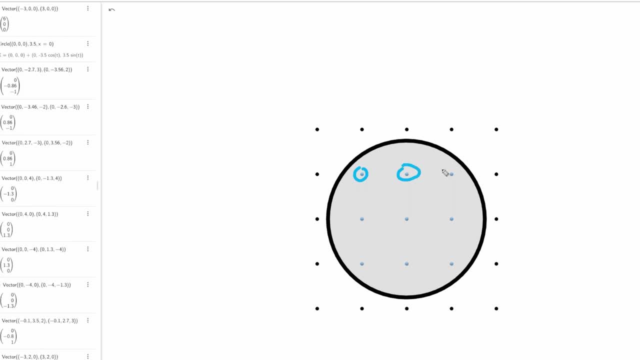 So what we do is like, hey, if it's an arrow pointing at you, we're going to draw like a dot with some circles around it. So here's some magnetic field piercing our hoop. but what we really mean is, like you know this right here. So that's a flux because there's arrows getting. 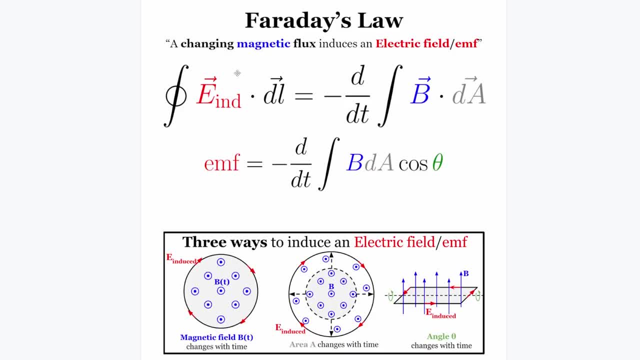 caught magnetic field piercing through that area. So what Faraday's Law says is: if you change this magnetic flux, if this thing changes, it's not enough to have magnetic flux. for Faraday's Law to give you an EMF or a field, You have to have a changing magnetic flux. So 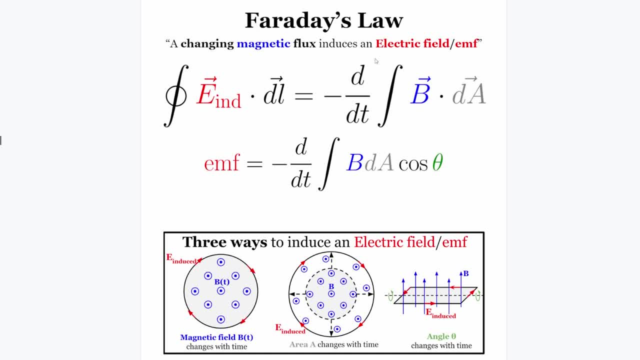 that's what this derivative here is doing. This derivative here stands guard and it watches over this integral, this magnetic flux. And this derivative is like: hey, hey, hey, hey. anybody in here changes in time, because I'm taking a derivative with respect to time, I'm making all. 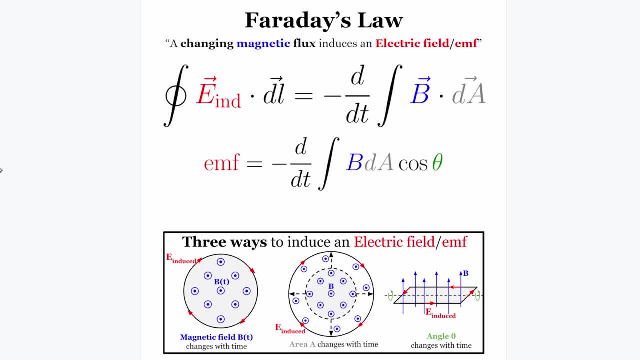 of this stuff over here. So that's what it does If it makes this stuff. what is this stuff over here? This is the electric field and it's also the EMF. You might be like I don't care about the. 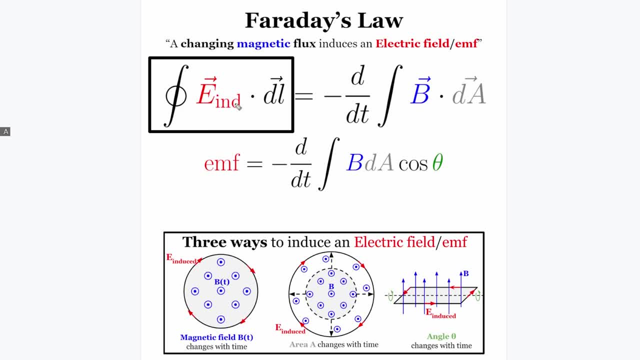 electric field? Yeah, most people don't. When you're doing Faraday's Law, a lot of times you don't care about the electric field. What you care about is that electric field times length has units of volts. So you're like, ooh, I do be caring about the volts because you know Ohm's Law says: 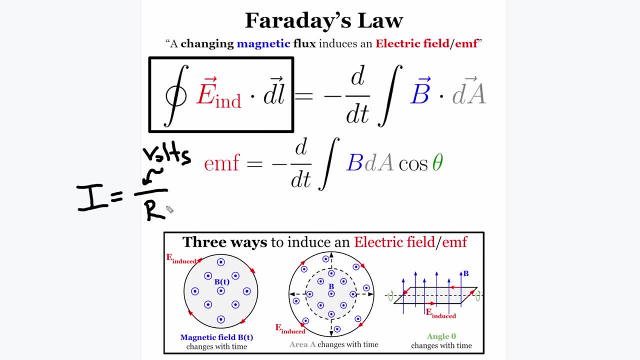 if you got volts, you divide that by your resistance and that gives you your current. So this has units of volts. but I have to warn you, this is technically not a voltage, It's not a difference in electric potential, because it's not getting created. This electric field is not getting created by a net. 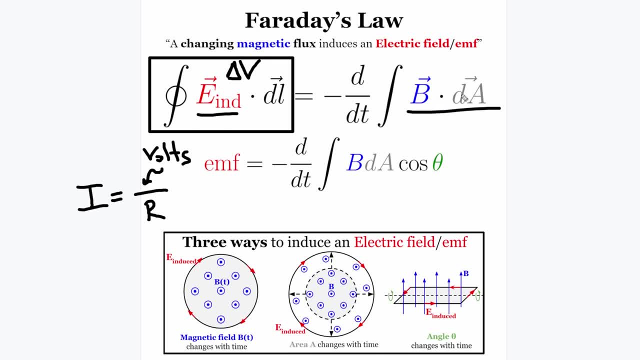 charge. It's getting created by a change in magnetic flux. This is what blew people's mind in Faraday's time, You know. he was like hey, Faraday was like, look, look, I can make an electric field. And people were like, okay, where's the net charge creating it? And he's like: 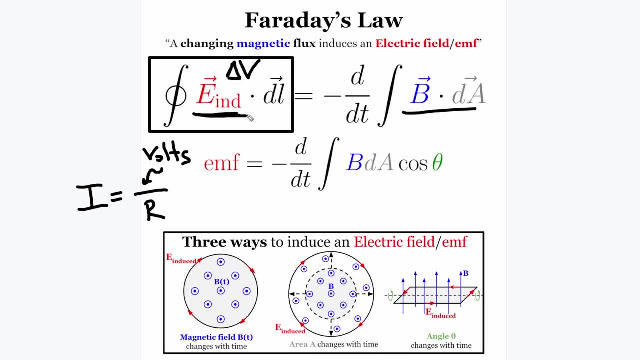 I don't have a net charge. I just changed my magnetic flux And this E field popped into the ether, like you know, like a magic trick, And they were like what? How can you do that? Well, because this electric field is not getting created by a net charge. 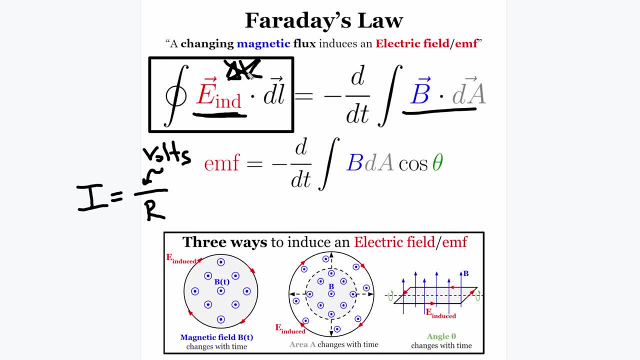 don't call it a voltage. Your professor will cringe if you say that It has units of volts. So this whole thing here in this box, it looks like volts, It tastes like volts, It smells like volts. You can plug it anywhere. that volts goes in all of your formulas and it works just fine. 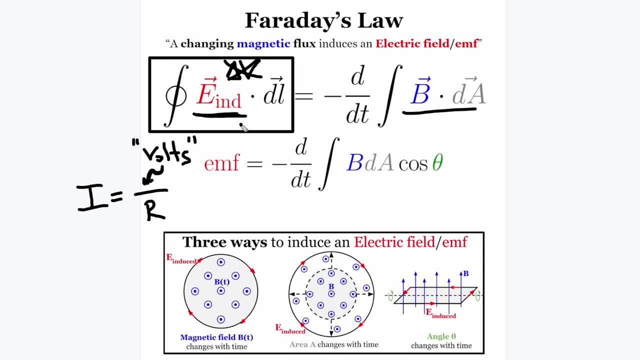 but it's not technically a voltage, So we give it a different name In the textbooks. you know you can think about it as a voltage, but in the textbooks they got to be proper. They call it an EMF, which is ironic, because you know, professor, be getting all uptight about me calling it a. 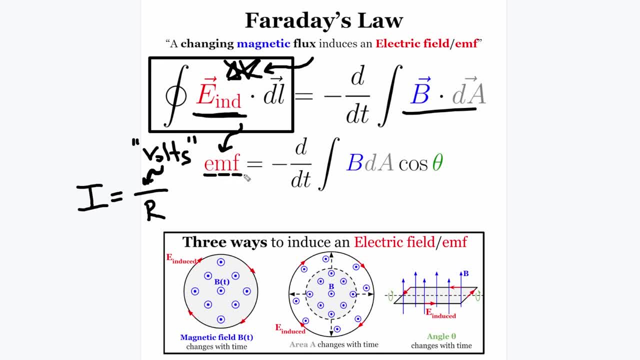 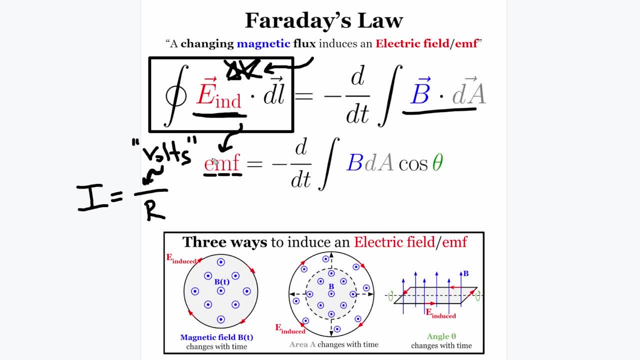 newtons. It's just a bad name. It's kind of a historical name, but it's got units of volts, So I'd rather call it voltage than EMF. but whatever, Everybody calls it EMF. but it's a volt, It's a number of volts. That's what we care about. So really, you don't do any of this integral. 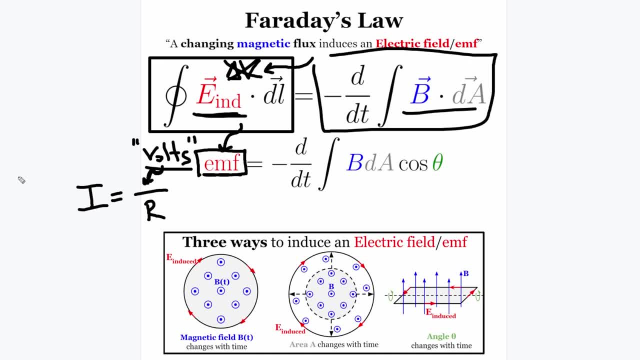 here. You just find this side and you say: that's equal to my volts, my EMF, And we care about that because that gets current flowing. So I just wrote this whole thing right here. The EMF is: usually I set it equal to negative d dt. You might be like whoa, but you wrote this different, Yeah. 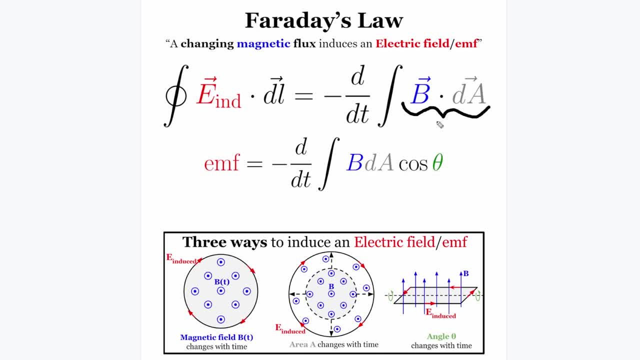 because, without loss of generality, you can always write a dot product as the magnitude of the one vector times the magnitude of the other vector times cosine of the angle in between those two vectors. So this is usually how you're going to deal with it. You don't really want to deal with. 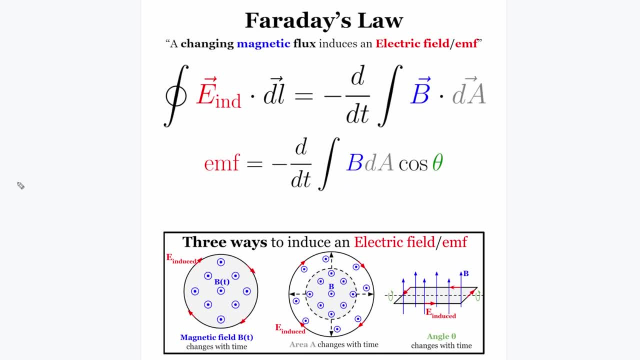 the dot product. Typically, you typically want to deal with it like this: This is the easier version than the top one I just showed you of Faraday's law, but it's still pretty gnarly. There's an integral here And you might be like: wait, I don't know what this angle means. What do you even? 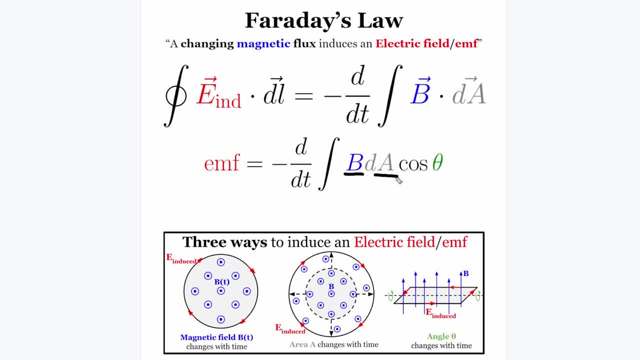 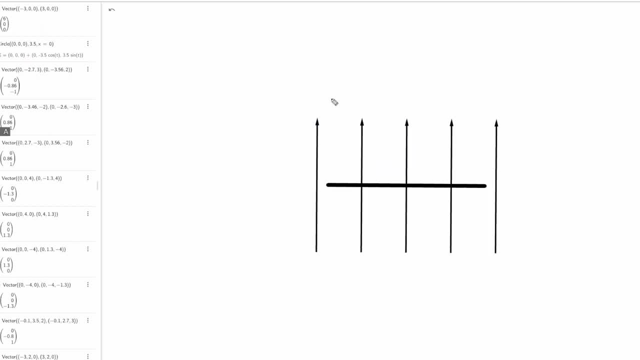 mean by that. So this angle is the angle between the magnetic field and the area. So in this case I just showed you right here You might be like: well, I know which way the magnetic field goes. It goes straight up. So I know that the magnetic field is going straight up. Which way is the area? 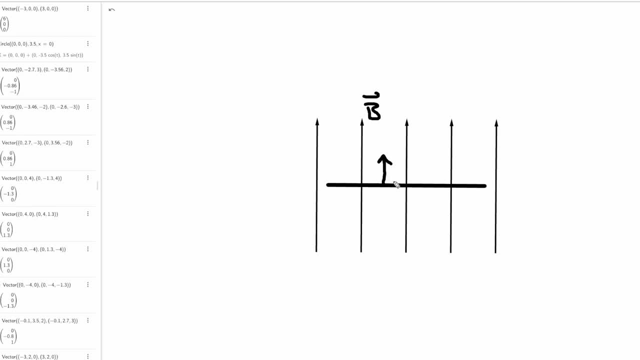 going. We define the direction of the area as this direction perpendicular to this face, this surface created by the area, created by this hoop, And you could write it as da, That's also the, So in this case B and da go both the same way, And so the angle between them is zero And that. 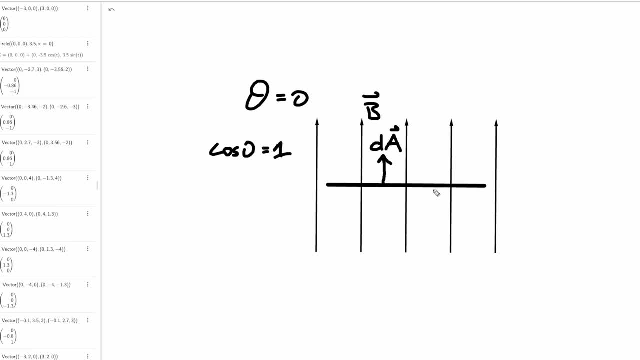 means cosine of zero would be one. This is the way you want to orient it. If you want to get magnetic flux, you want to orient it like this, Like if you go jellyfishing- you know your SpongeBob jellyfishing, this is how you want to hold your net. Look at all that. Look at all that flux. 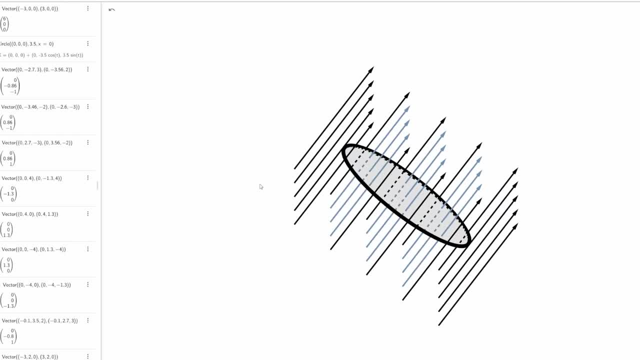 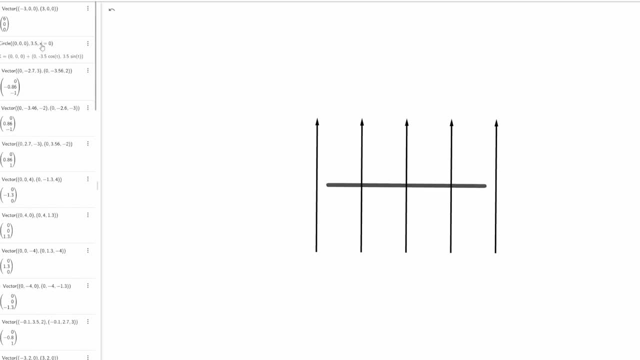 piercing your hoop. If this was like a net, look at all the jellyfish flying through your hoop. There's a lot of flux. You want that B pointing in the same direction as your? da You could. you know you don't want to do this. You don't want to be. 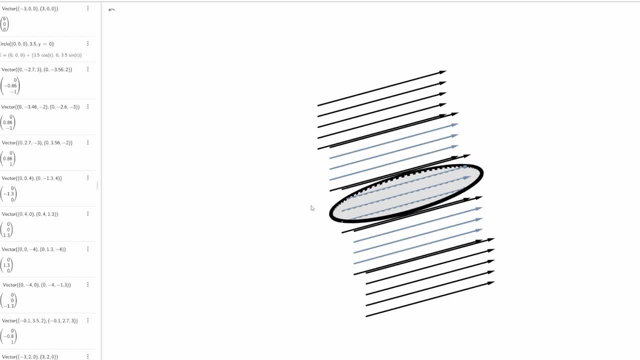 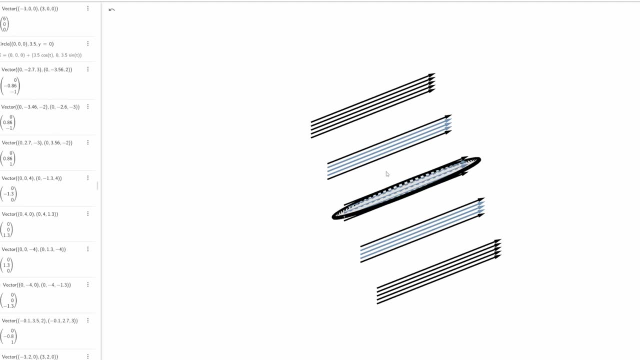 you know, squidward over here pulling one of these jams, It's like, oh dude, you're not catching nothing now Like it looks like you are, but all these field lines are just glancing the top of your net. None of them are actually piercing through your net. You can imagine. 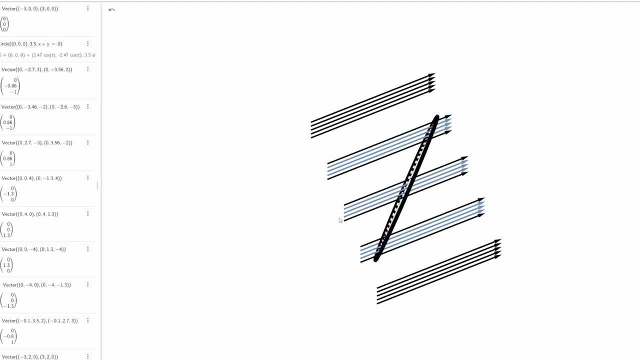 intermediate angles where you have like something like this: All right, at least you'd be catching something. You know this isn't perfect, but at least you're catching something. So in this case, your area vector would point this ways right here, you know, perpendicular to the face of your area. 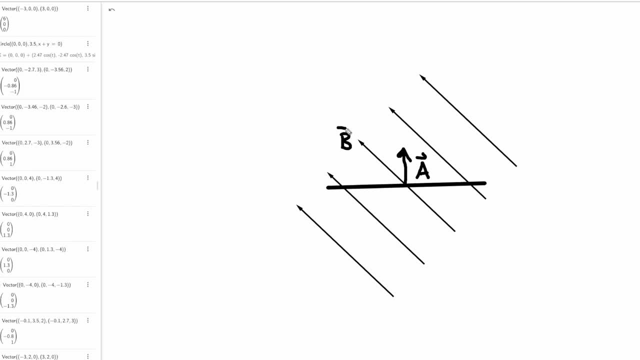 That's the A or the DA, whichever one This way is B. So these, these are external magnetic fields getting created by something. here. This is the direction of the magnetic field And that angle is this right here. This here would be your angle that you want to find. So when I write BA cosine, 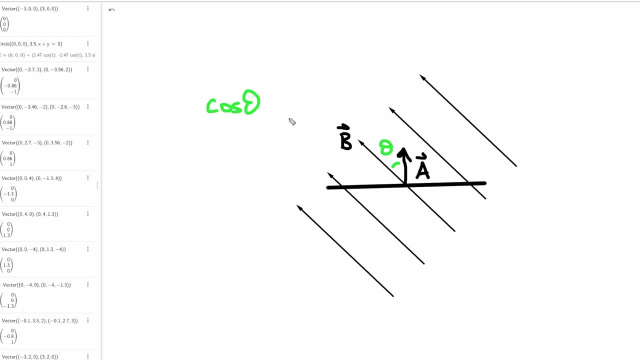 of theta. I'm talking about this here. That's what that cosine of theta is, You might be like. why is it that theta? Well, look, the only part of this magnetic field that matters, that creates flux, is the one going through the hoop. So look, this B field here, the only part of it that matters. 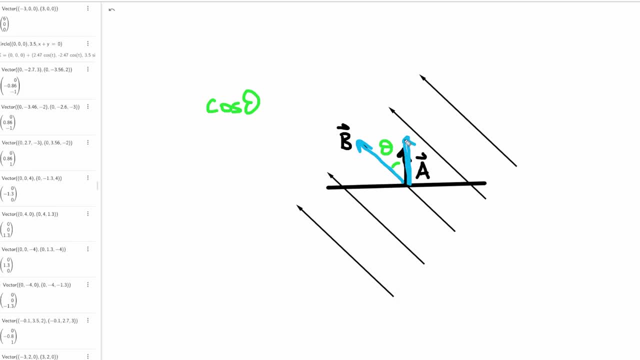 this ways. So that's why I want to do cosine theta. Look, this piece here is the adjacent part of that hypotenuse. So I want to take cosine of theta to get this piece. This piece doesn't give me any flux, It's just this piece. That's why we have that cosine theta right there. So you get this. 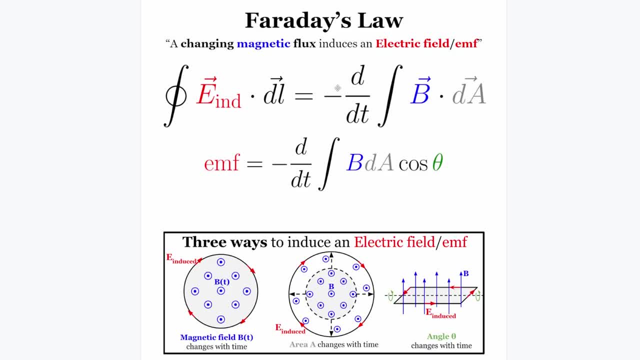 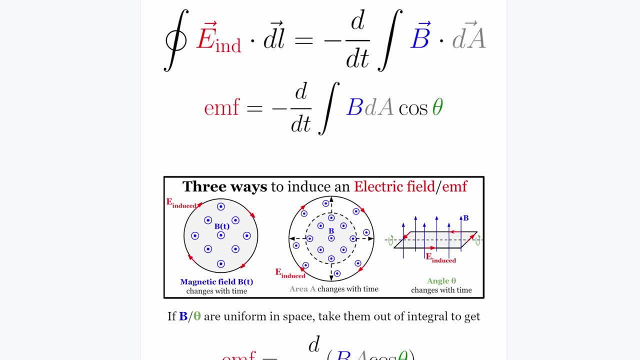 formula here. It's a little better for Faraday's law- And you're like: okay, well, how do I actually do this? If I wanted to actually go to the lab and change the magnetic flux, what would I do? You got three choices, because there's three things in here: There's B field. there's area. 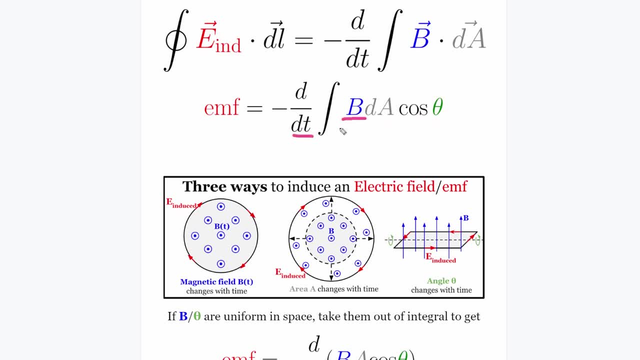 there's theta, So you can either change- you know DDT, change in time, the magnetic field. So maybe this magnetic field gets more and more intense, you know it gets stronger or weaker, or you change the area, Maybe. 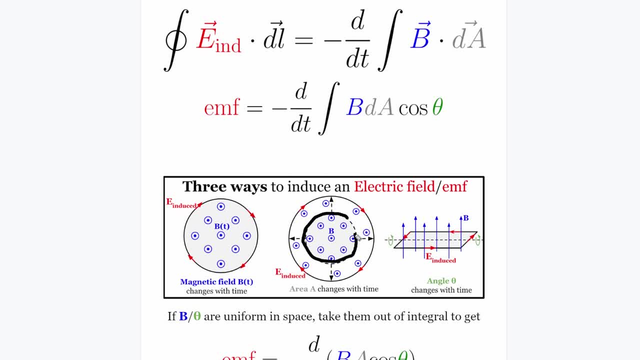 your area was small at first. you had a small circle and then somehow it can- like you know, the metal can slip past each other and you get a bigger area. you're catching more flux. That's another way to change the magnetic flux, or you change the angle. So maybe you have this rectangle. 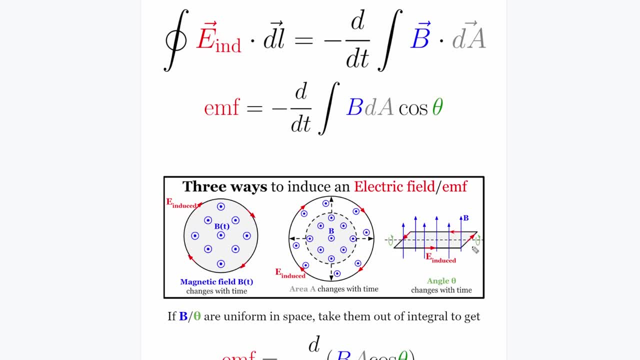 and you just rotate it in a magnetic field so that that angle you're creating here is changing in time. So that's another way to change the magnetic flux. That's the third way to do it. Those are the only ways to change your magnetic flux. And if you do, 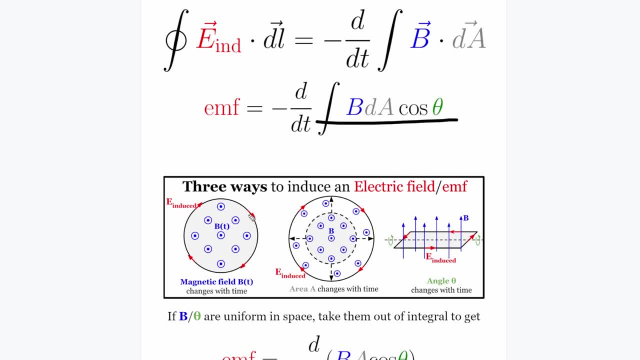 that you'll get volts, which means a current will start to flow. Okay, so this is still, honestly, more complicated than what you'll usually have to do, So you can simplify this even. you can simplify this even more And you can say: well, shoot, if my magnetic field is uniform, what does? 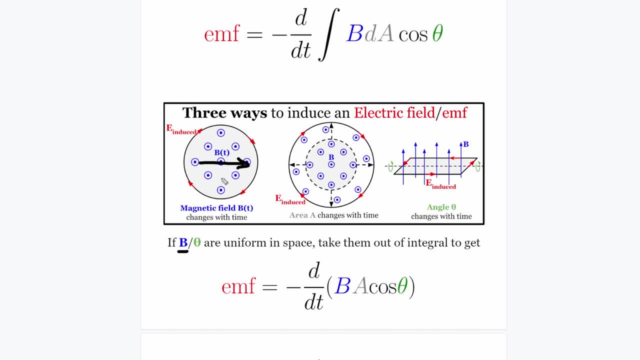 uniform mean It means the same through space. So the magnetic field doesn't change when you go that way and it doesn't change when you go this way. So in space the B field is uniform. if that's the case, This integral only cares about space, like this integral over space. So 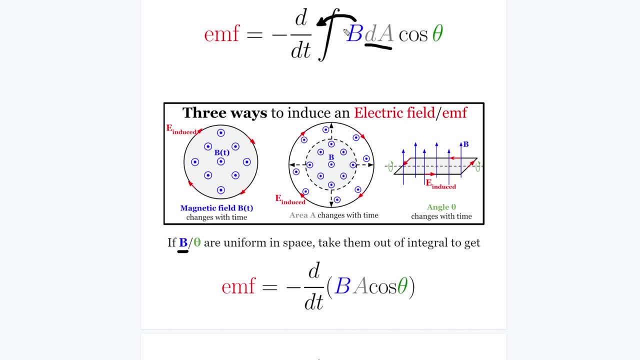 if your B doesn't depend on space, it gets to get smuggled out of your integral, even if it's time dependent. you can just come out of this integral, That's cool. And if your theta doesn't depend on space, like if your angle is always in the same direction, you know, for this example we had up 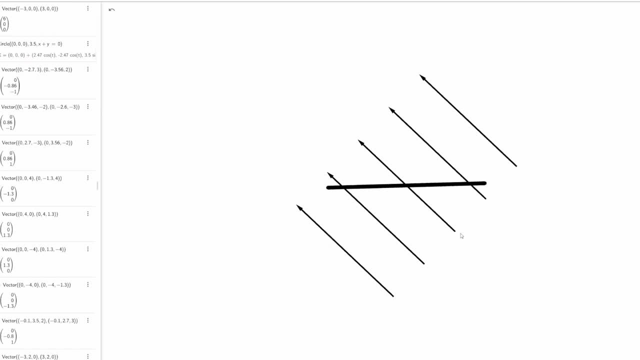 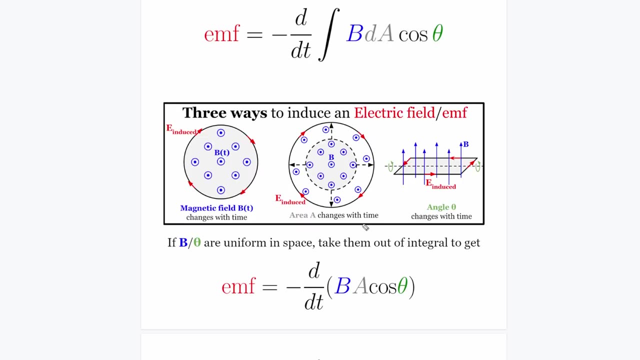 here. if our angle is always like- even though there's an angle, it's always the same angle all the way through it's uniform- you can smuggle that out of your integral And that can just come out front And what you'd be left with is: think about it. you'd have negative d dt. we smuggled B out, we. 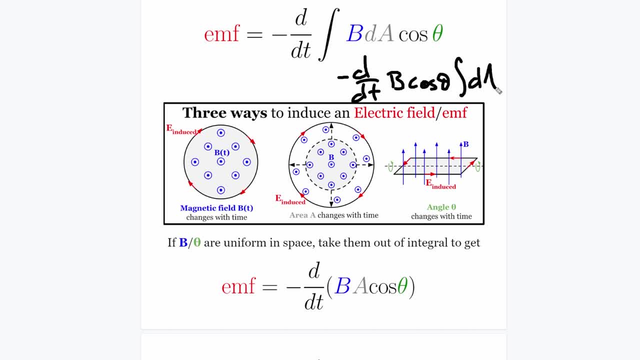 smuggled cosine theta out, you'd just be ended up with integral da. But the integral da is just a, so we take this, we just call that a. this is b, that's cosine theta. we just end up with this formula right here, which is the simpler version of Faraday's law: If, if the magnetic field is 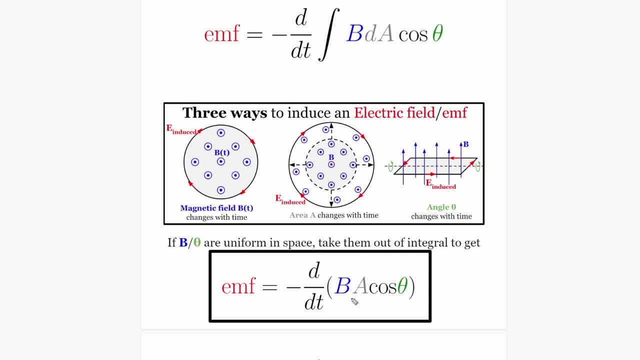 uniform in space, you know, same throughout space. then you can use this easier version right here, which is kind of nice. When wouldn't you be able to do that? Well, if B is not uniform, what would that even look like It? 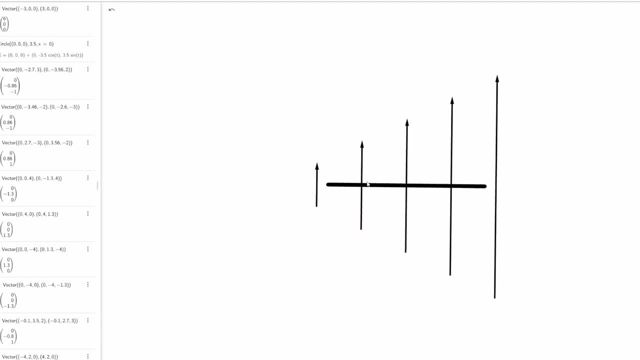 would look like this: Look, here's a magnetic field that's not uniform in space. Look, if I move to the right, my magnetic field is getting more and more intense. I'm representing that with longer line arrows. The other way you could represent it from this direction you can't really tell. you're like 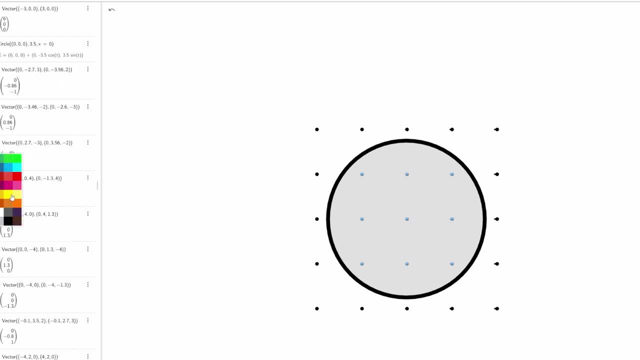 dude, I can't tell if it's getting more intense. So a lot of times what we do, you know on a page that's not 3d, First of all we draw these little circle around them because, like if the arrows, 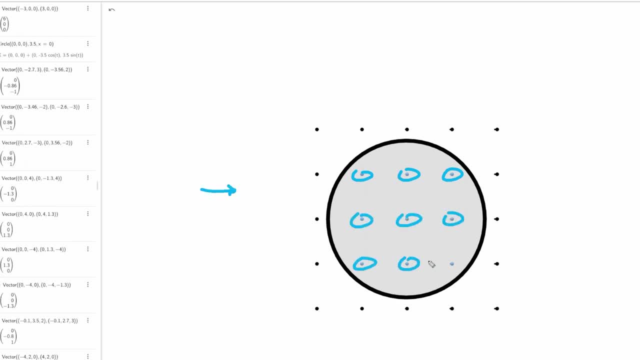 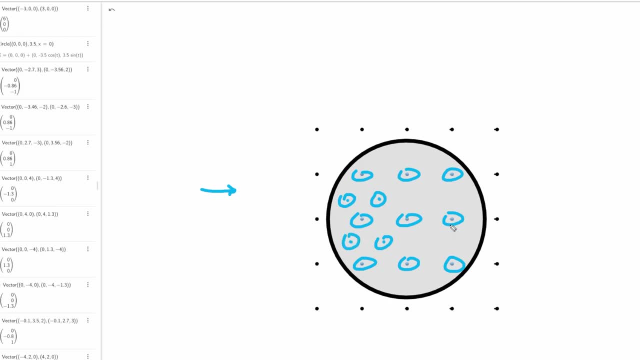 these. So this would be a magnetic field that's more intense here on the left than it is on the right. it'd be a non uniform magnetic field, or the way I had it drawn earlier. more intense on the right means there's more of these arrows coming at you on the right, So that'd be non. 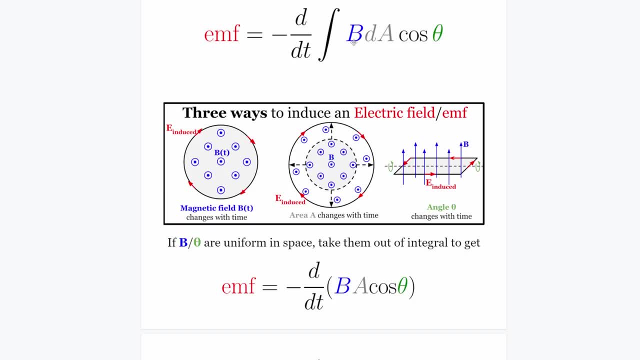 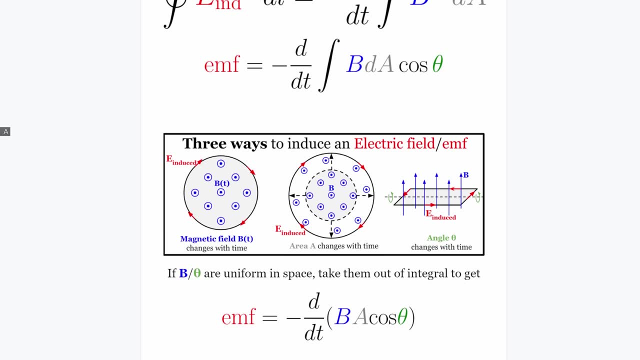 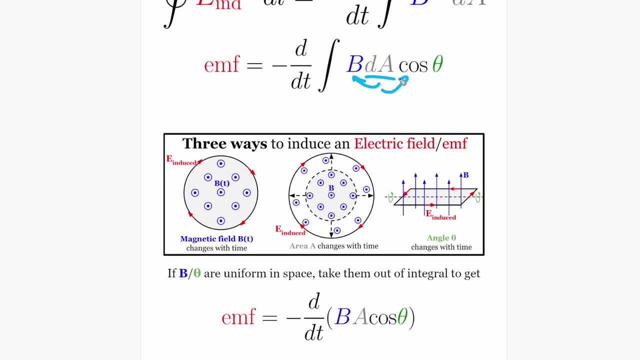 da is always watching this. da is like, hey, hey, hey, anybody in here depend on space. I'm going to integrate you And you have to leave the stuff in there, But if B is uniform, you don't have to do that. So let's try some examples. How do you do this, Well? well, one thing might be bothering. 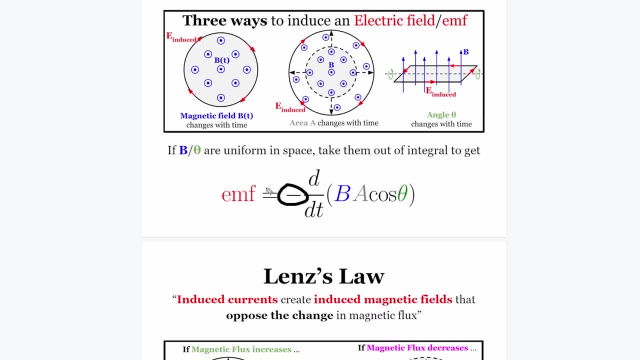 you might be like: what the heck is this negative doing out here? Okay, there's a whole story behind that. I'll get to that in a minute. I don't want to bore you, though. That's Lenz's law, We'll get. 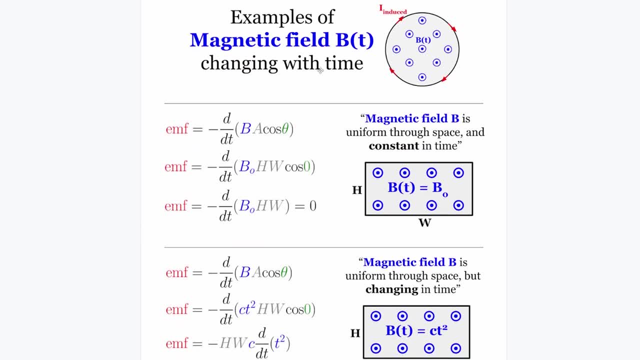 to that. Let's just first do a couple problems. Let's kick the tires. So there's three things you could do: change the magnetic field, change the area, change the angle, for example, if you want to do some examples where we change the magnetic field. So here's an example: we got a magnetic 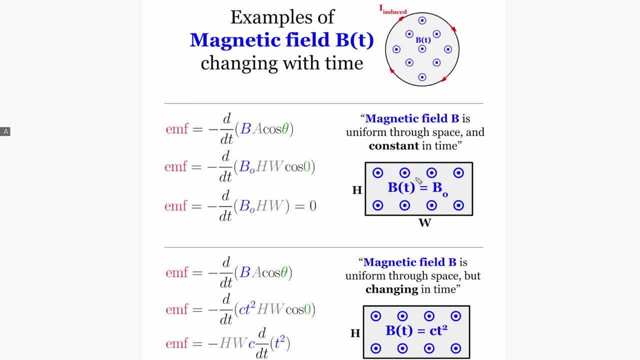 field piercing this rectangular hoop. So we got a flux. look, we got a flux here, So I can use the easy version, because this magnetic field is uniform through space. it doesn't vary vertically or horizontally. it's the same value throughout space. So we get to use this easier version of Faraday's. 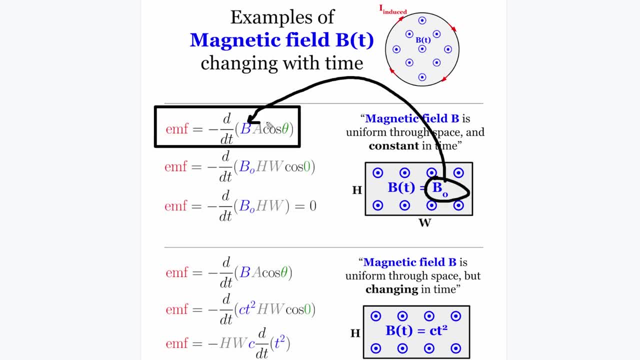 law And the way you do it is: you just find what your B is, throw your B into there, find what your A is, but that's just height times width. you know how to find area, find your angle, but you know. 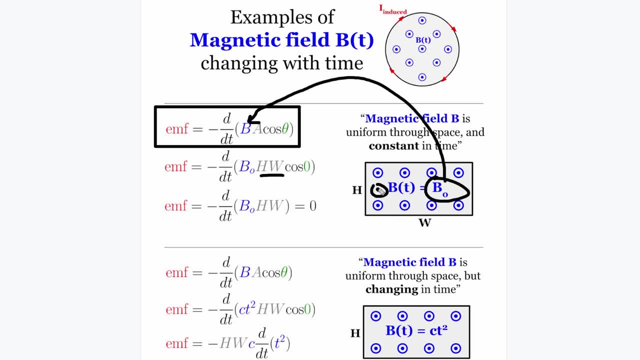 the surface area. here you know how to find the area. you know how to find the area. you know how to find the area. here the area points straight out, the area vector B point straight out. so it's cosine of zero, and cosine of zero is one. So that's good. But then you always got this derivative. 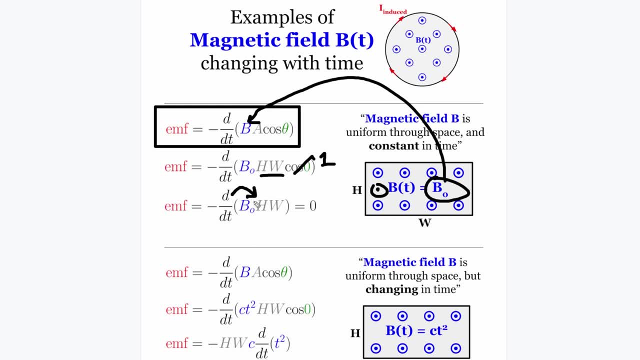 out here lurking. this derivative looks inside like hey, anybody here changing time? And they're like: No sir, no sir, no ma'am, Okay, well, shoot, you annihilate all you. I do take a derivative of a constant, I get zero. So in this case, even though you had a flux, you get no EMF, no volts. 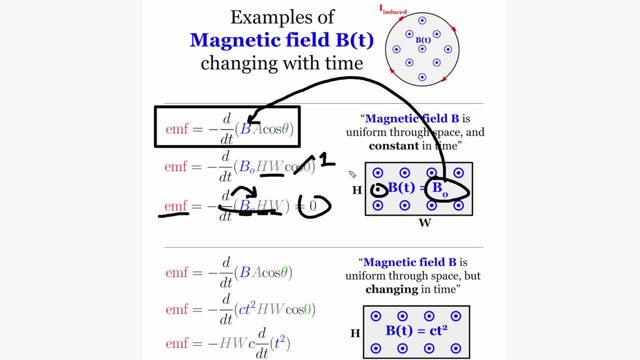 for you: no currents going to start flowing here because there was no change in that flux. It's not enough to have a flux, you have to have a changing flux, So that one's kind of easy. you know, you might get tricked on a test. you might be like hey. 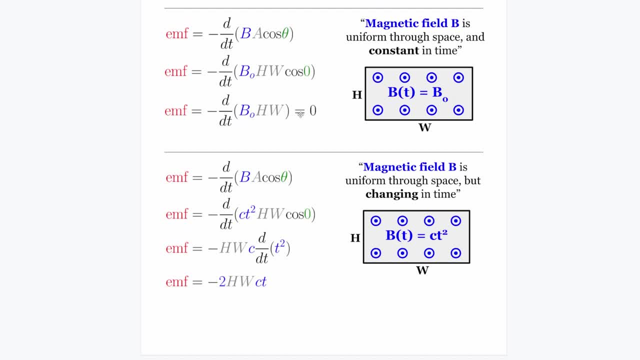 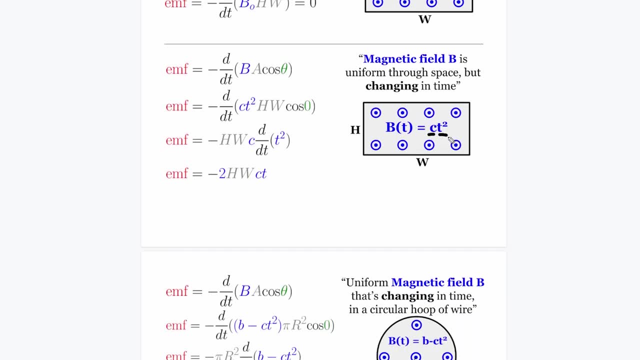 real complicated setup. But if nothing's changing in time, it all gets annihilated, And so you know EMF. All right, what if you do have something changing in time? here's a magnetic field changing in time. we got some constant time c squared, so it's getting more and more intense. 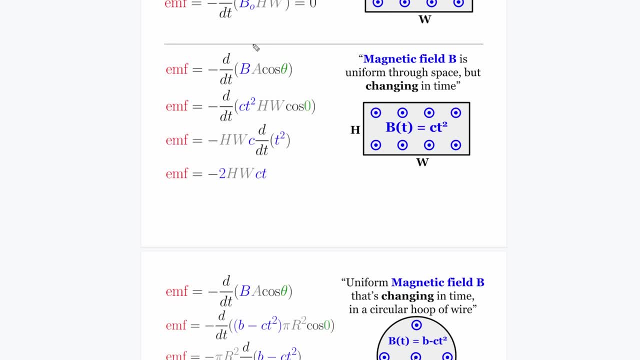 As time increases I get more and more magnetic field. But I don't have to do my integral version because this B field gets uniformly greater, like it gets more on the right and on the left at the same time and in the middle, So it's not like a function of space. So I get to do my easier. 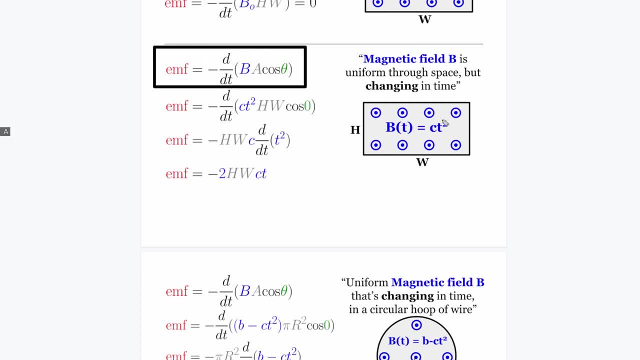 version of Faraday's law, And what I do is just plug in my value. I plug in my what. my B is constant times t squared. that goes there. That's why I have this. you know how to find area, height, times, width, the angle- still nice, and cosine zero just gives me one. All right, so I got all that. 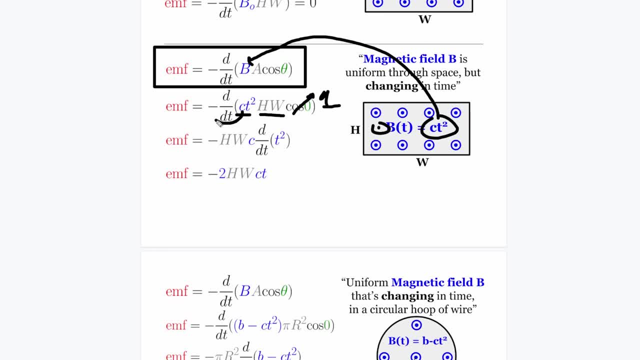 my derivatives now like: hey, hey, hey, hey, C. do you depend on time? Nope, Okay, you can get out of here. HW- depend on time? Nope, you sneak out the back door. all that's left in there is the. 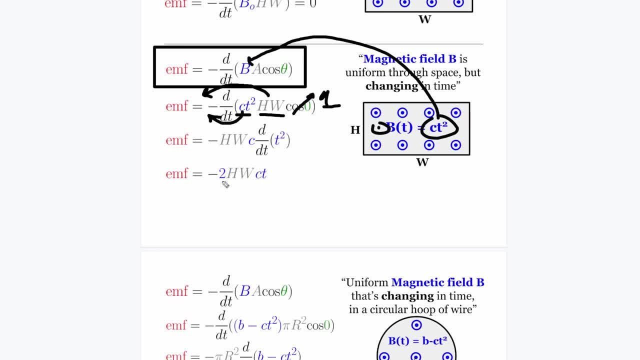 t squared, But the derivative of t squared is just two t, So the two comes out. I get two hw ct is mf. the number of volts would be this: So if I wanted the current that flows, I could take the number of volts to hw ct and then divide by. if I knew the resistance of this circuit, I could just 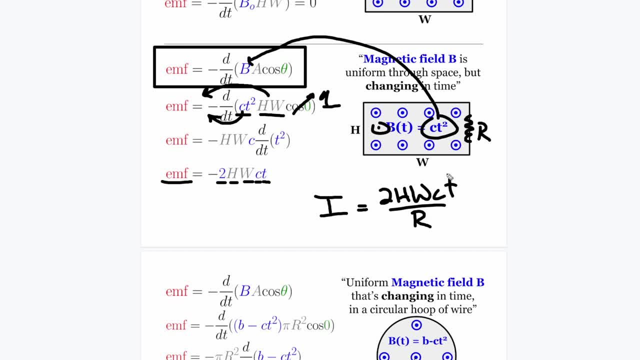 divide by the resistance. But which way does this current flow? That's the question. That's what this negatives here for And I'll be honest, almost everyone that does these problems just finds the magnitude of the emf. they just make it positive And then they have a different way. 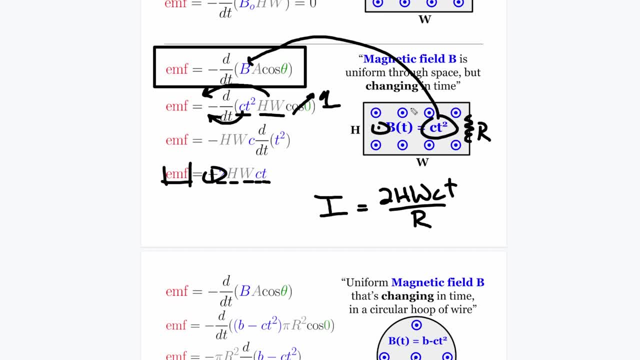 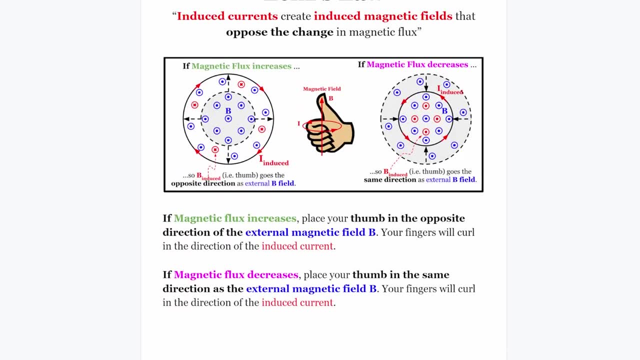 to figure out which way this current flows. Does it flow clockwise, Or does it flow clockwise? Does it flow counterclockwise? So there's a rule to figure this out. That's what that Lenz's law was up above. So how do you figure out which way the current is going to flow? Lenz's law says that. 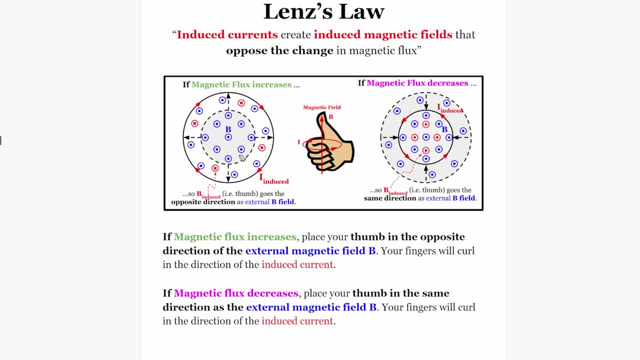 wires hate a changing flux. they want to keep their flux. whatever it was, they want to keep it. So this wire here had a small amount of flux. then you increased it and this wire was like, ah, dang, heck, no. So you increase the flux, you get all this new field coming out of here. 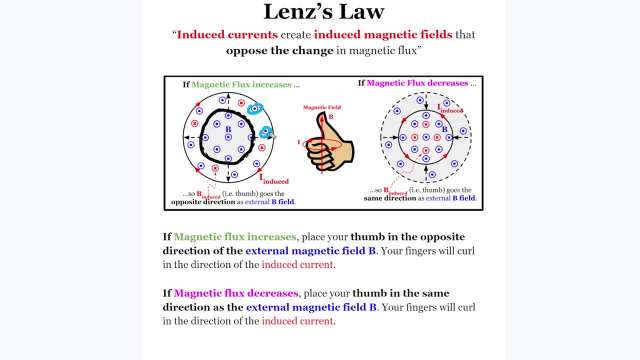 So this wire is like: okay, I'm going to pose you, I'm going to fight the change. So it starts that fights all this extra tries to delete them by making magnetic field go the other way. That's why I have these X's here. These X's are representing the induced magnetic field. 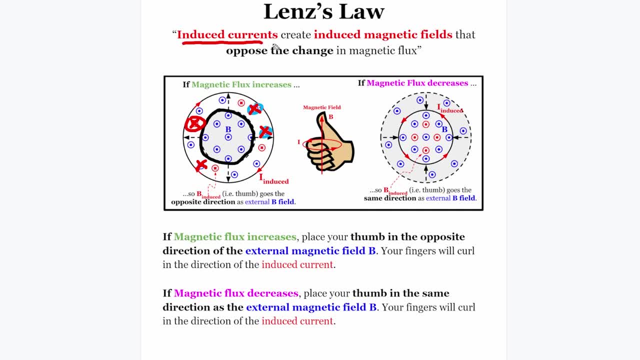 What is inducing the magnetic field? a current is, so current is going to induce a magnetic field. This is not the external magnetic field. like this blue is an external magnetic field created by some other. you know magnet, but a current is going to flow in here And the way you figure out which? 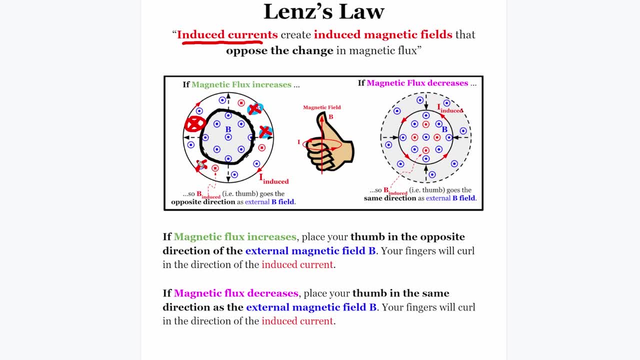 way that current flows is. you figure out which way would you point a magnetic field to fight the change? So I'm going to fight this increase by having magnetic field into the page. And now we use the right hand rule. So this right hand rule, 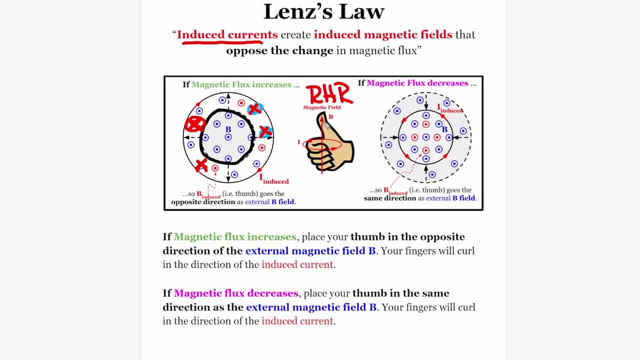 says, if you got a magnetic field into the page in the direction of your thumb, your fingers will swirl in the direction of the current needed to create that magnetic field. So try it right now: stick your thumb sort of in the direction of your screen and your fingers are going to be. 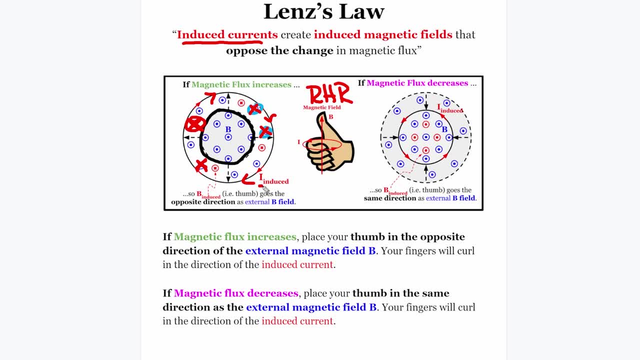 swirling this way. That's why I draw these arrows this way. That's the direction of the induced current. So what happens here is: you got a hoop mind in its own business. there's no current. you boost the flux by increasing it and this wire is going like no way. I don't like that. So it creates a current. 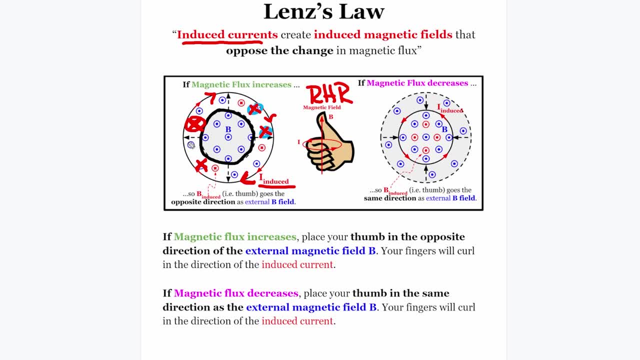 the current that flows is from that induced emf And it flows this way in order to fight all these extra magnetic fields. it's not going to win, you know, it's always going to lose, but hey, you know, it tries hard, it tries to fight this flux. it doesn't. it doesn't actually succeed in. 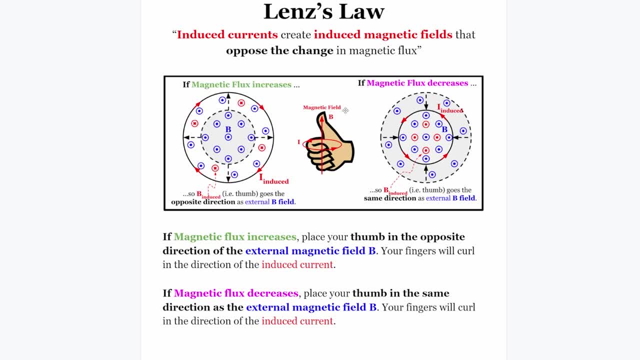 doing it, it can't cancel all of it, typically. Okay, what's the other example? Well, let's say you decrease the flux. So if you decrease the flux, if, if you had a hoop that was this big and you go back to what it was, 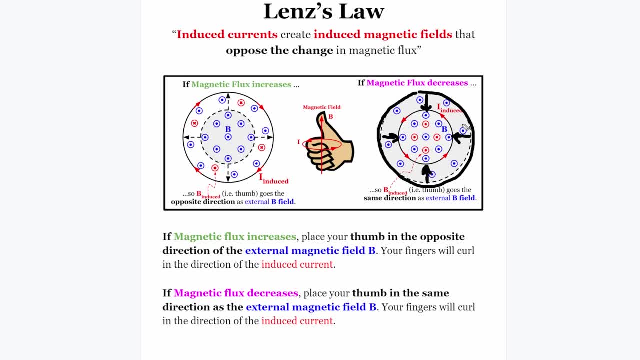 I think, oh, it's going to be happy now. No, this hoop has no memory. It's always fighting what you did. Now it's going to be like: oh, I liked this large amount of flux, I want to keep it. It's. 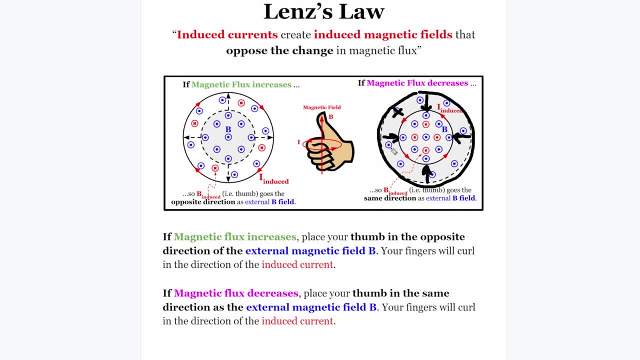 always trying to keep whatever it just had. You're like, well, you got rid of these. No, no, no, I want to keep these. You just got rid of them. I'm going to try to put them back. It fights the. 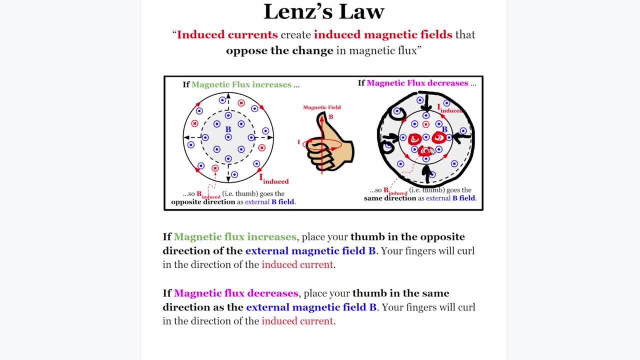 decrease by trying to put them back. That's why I drew these induced magnetic fields going in the same direction as the external magnetic field. So which way should the current flow? to do that? Well, take your thumb, put your thumb in the direction of this out of the page and you'll. 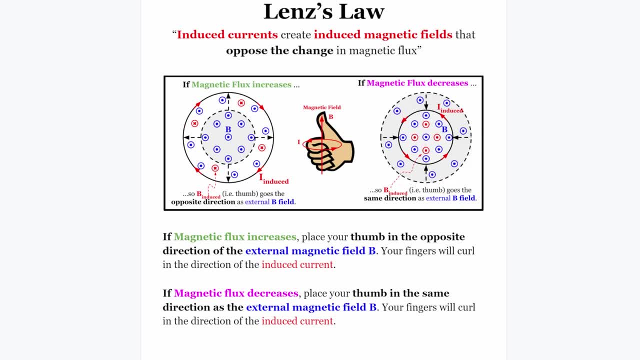 realize your current should flow that way in order to do it. So I got it written down here. You can read it if you want. I'll share this document in the comments. But you know, if the magnetic flux increases, put your thumb opposite the external magnetic field, your fingers curl. 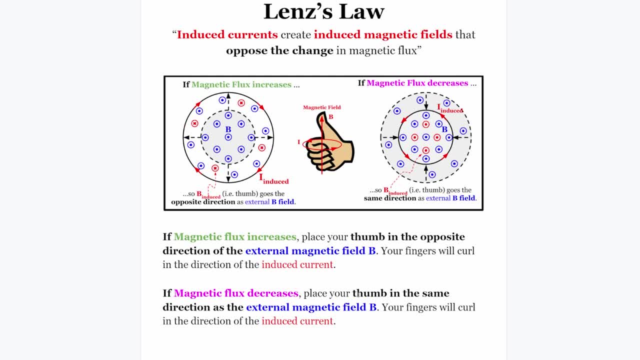 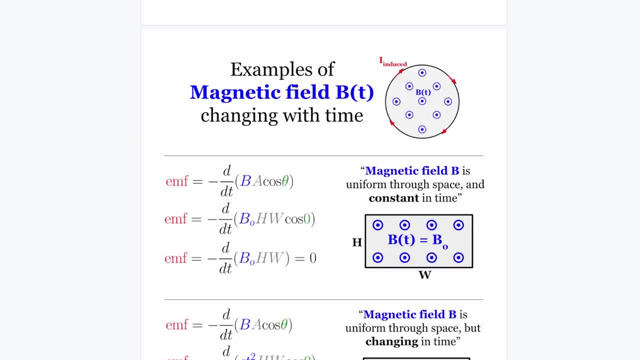 in the direction of the induced current. If your magnetic flux decreases, place your thumb in the same direction as the external magnetic field and your fingers curl in the direction of the induced current. So let's try it out. What did we find here? So the first question you ask is: 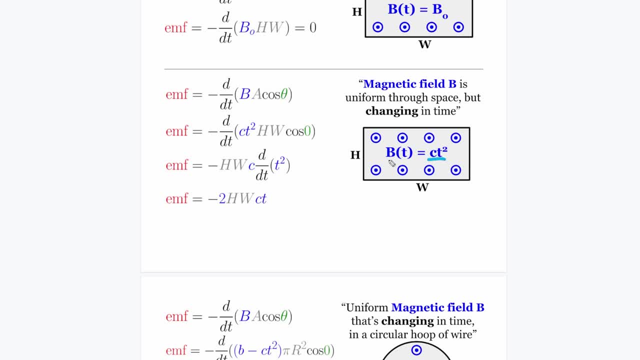 was flux increasing or decreasing. Well, look, as time increases, B is increasing, So we're getting more and more magnetic flux in here And our hoop's going to be like: oh hell, no, I don't want that, I want what I had. So I'm gonna try to get rid of U. 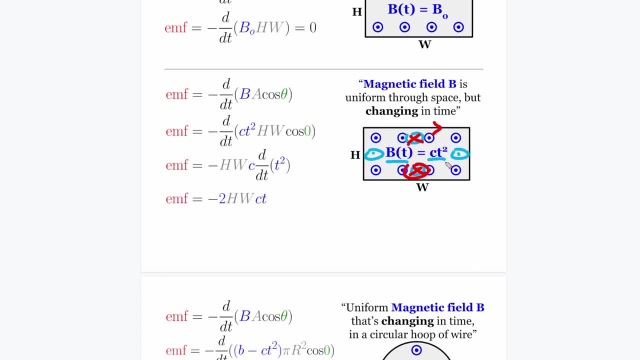 So it creates an induced magnetic field into. put your thumb into and you realize the current's going to be flowing in this clockwise direction. That's why you typically don't care about that sign. You just find the magnitude of the EMF, You figure out the direction of the induced current. 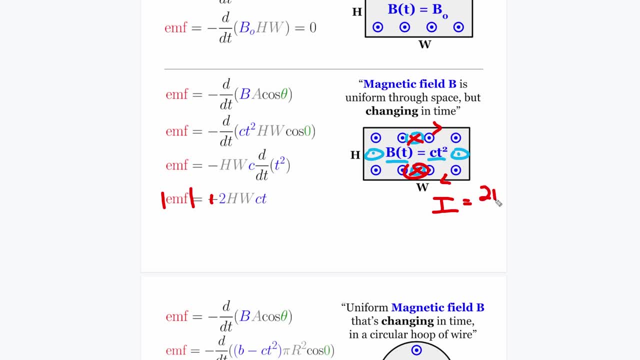 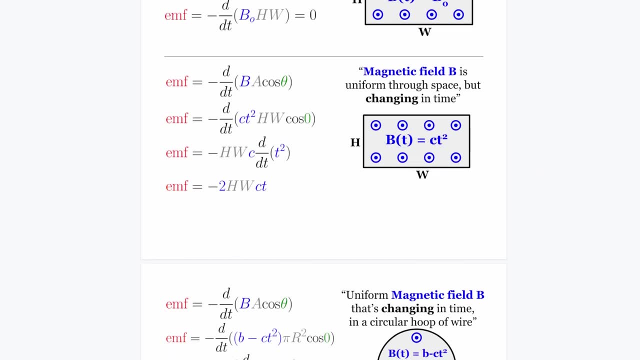 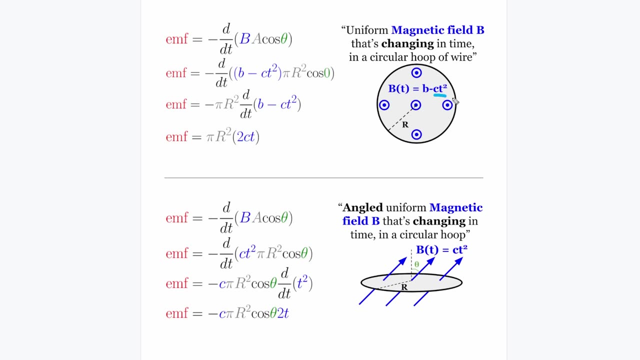 separately And again the current would be whatever that EMF was. you know, 2HWCT over this circuit was Okay. so that was an example of Faraday's law. Let's do another one. What if you got a circle and the magnetic flux is decreasing this time? Look, I'm subtracting as time increases. 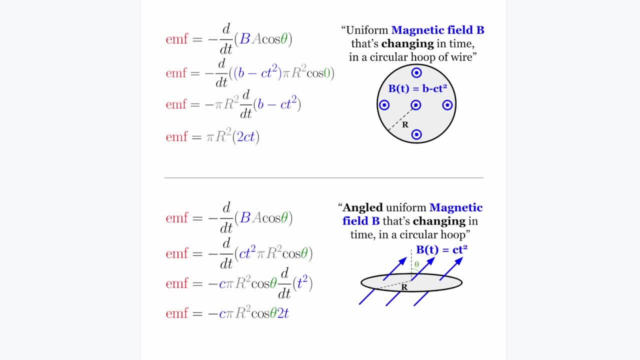 So I'm subtracting flux that's coming out of the page. So well, same thing. B is uniform. So if B is uniform, we get to use the easy version of Faraday's law. We're going to take this B. 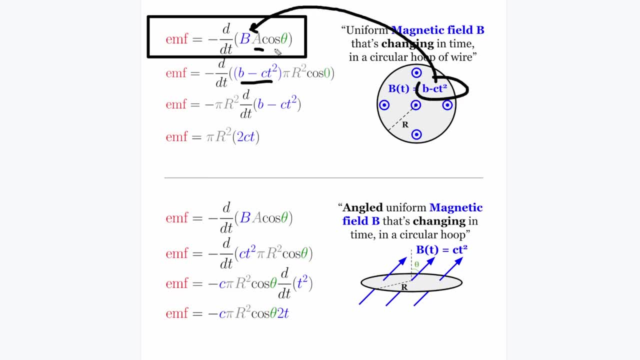 whatever it is, and we're going to put it in for B, That's why I have it written here. We take the area. You know how to find the area of the circle, pi R squared And the angle's all nice. 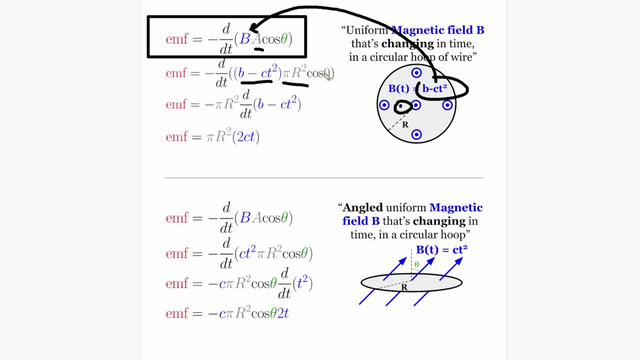 Area of the, the direction of the area and the B field point the same way. So cosine of zero is just one, All right. And then your derivative's sitting here waiting. It's like: hey, hey, hey, I'm going to operate on you. You depend on time, Pi. no, I don't Sneak out front R squared. 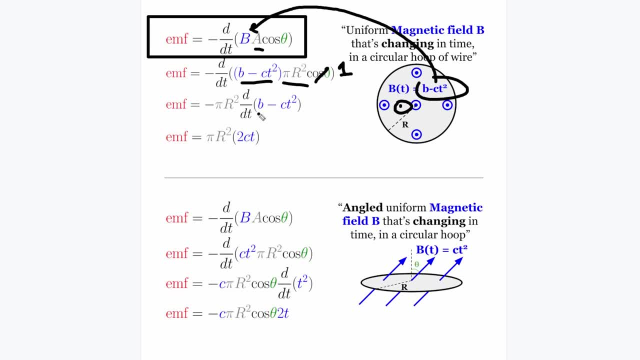 no, I don't Sneak out front. That's why they go here. So it's going to take a derivative of this here. but B is a constant. We're assuming B and C are constants, So B is a constant You get. 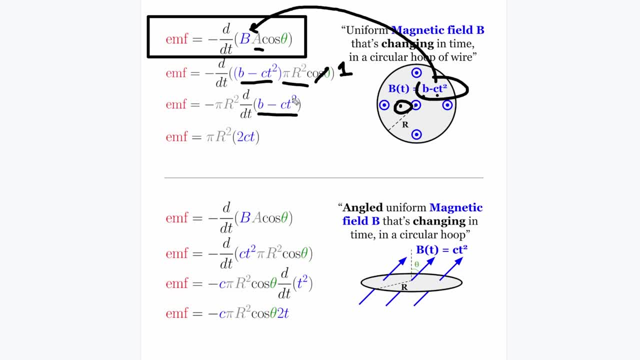 annihilated. So I get the derivative of negative CT squared. That'd just be negative of 2CT. So the negative got canceled here. but it doesn't matter, Cause we're going to figure out the direction of the current separately. So if I wanted the 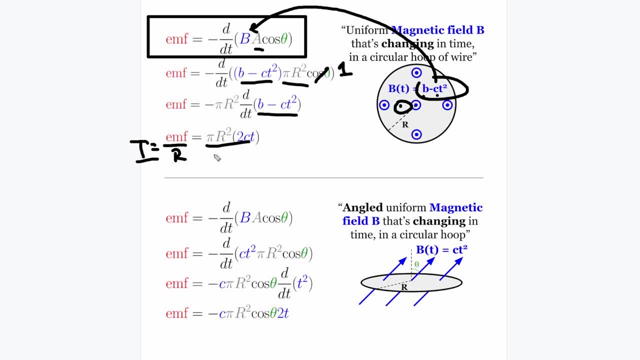 you know the current would be, whatever the EMF is over R. And again, be careful, I'll use little R, little R for resistance, little R, not capital R, like radius. This would be the resistance of the circuit And you'd figure out which way it flows using Lenz's law. You'd be like: all right. 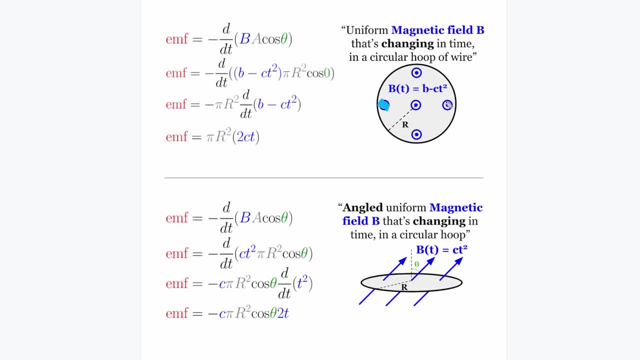 does my flux increase or decrease? This time it decreases. You're like deleting these. It's like, oh no, So this wire is like: oh no, I'm losing my flux, I want it back. I want to keep the same. 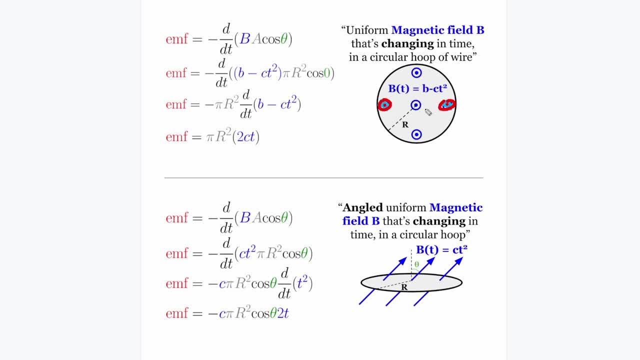 amount I had, So try to put it back. So now you stick your thumb thumb in the same direction as the external magnetic field. This is the induced red magnetic field, and your fingers will curl this way. This is the induced direction of the current. 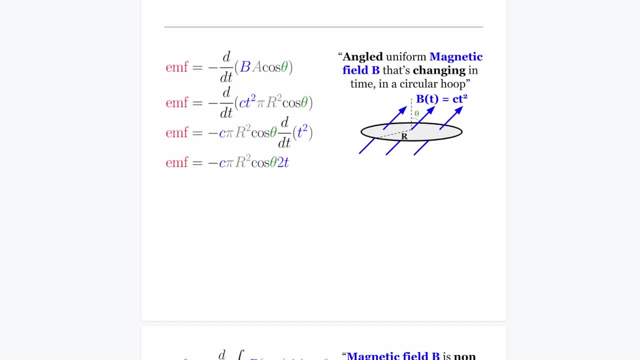 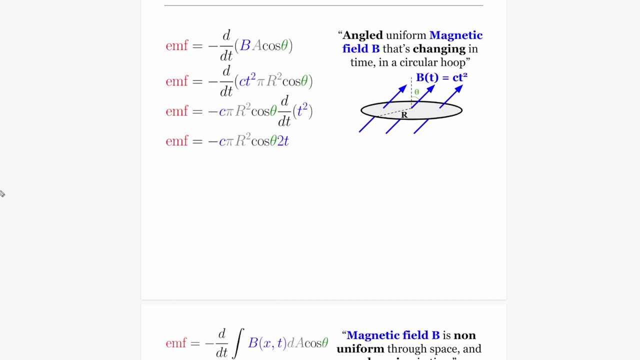 So that was an example where flux decreased. What if the angle's important? So that's how we've got an angle going through here. That's okay. Magnetic flux is still uniform. So we get to, you know, do the easy version of Faraday's law, We do this version right here. We take our B field. 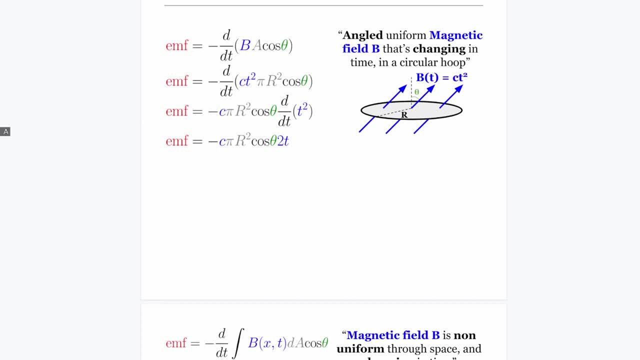 whatever it is, take CT squared And we take this and put it into B, So I take CT squared Area's still pi R squared, But this time we just we have a cosine theta that matters. We need cosine theta because we need only the part of. 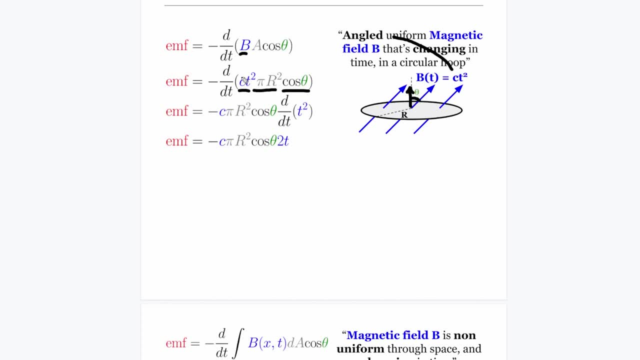 B that goes through that hoop. So I got that. Everyone can sneak out, All y'all can get smuggled past the derivative, except for T squared. The T squared is going to have to take a derivative, So I get two T out of that And so I get my EMF. is this, And again you can do. Lenz's law Does. 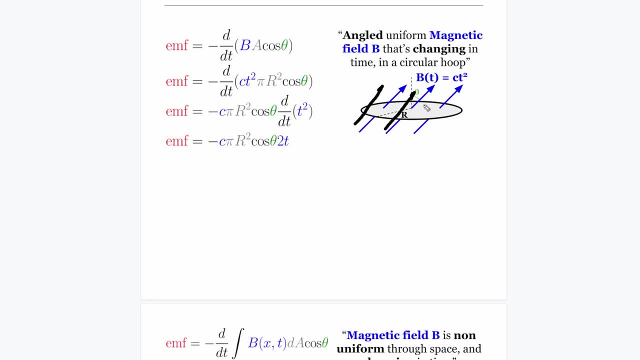 flux increase or decrease. It increases- We're like increasing how much B goes through here. So our hoop's like: oh heck, no, I'm going to try to get rid of you. It can't create an angled one, but it can create a down one. I'm trying to fight you. Put your thumb down. You realize okay. 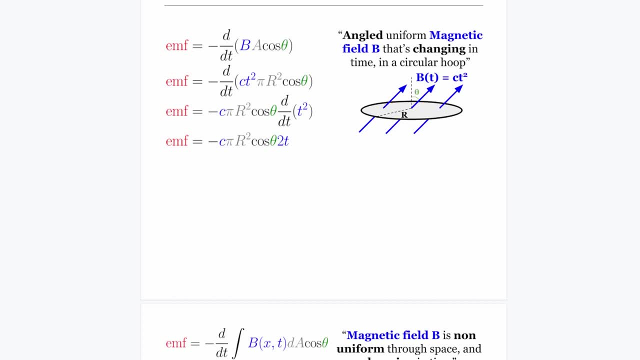 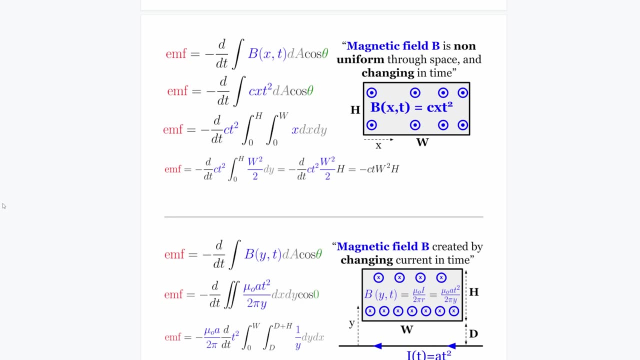 current will be flowing around that way. So that's another example. How does this get harder? Okay, What if you had a magnetic field that actually was non-uniform, That is to say, if you head out in the right word direction? what if you do get more and more magnetic field that way? You know? 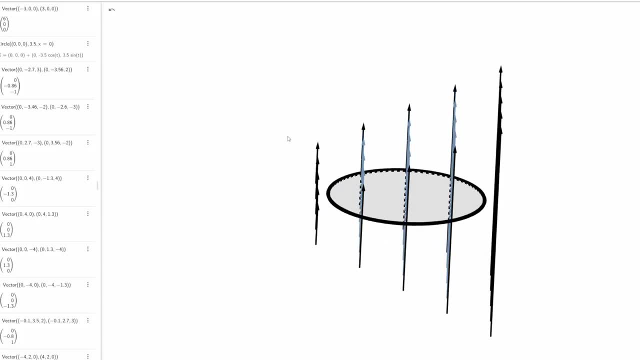 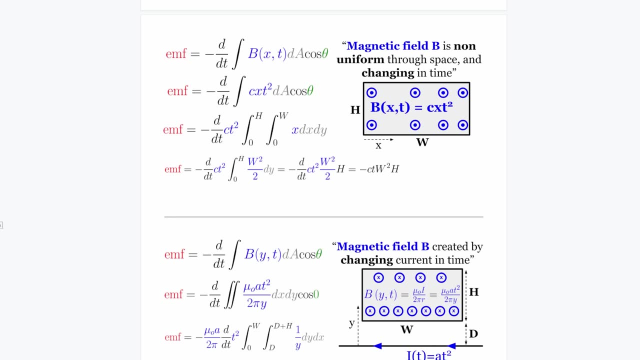 that's like. this is like this example right here: Non-uniform magnetic field. Now you have to do the we're going to have to integrate. We can't smuggle B out of this integral, because this, this integral DA is like Hey, Hey, Hey, anybody here depend on space? And the B is like yeah. 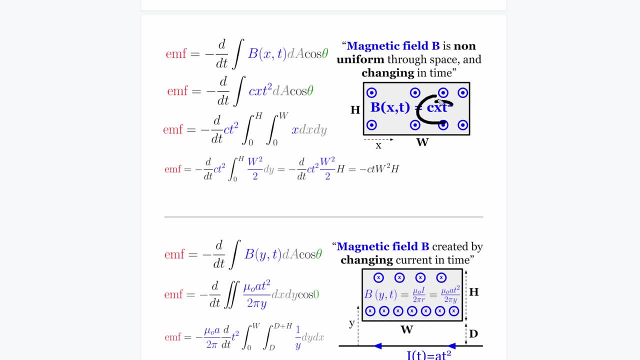 I do look. I depend on X. So you take whatever you take, your B, you throw it in here. That's why I have C, X, T squared. integral DA- at least our angle between area and B is still just cosine of zero, So it's one. So let's see, can anyone get smuggled out of the integral C? can that's? 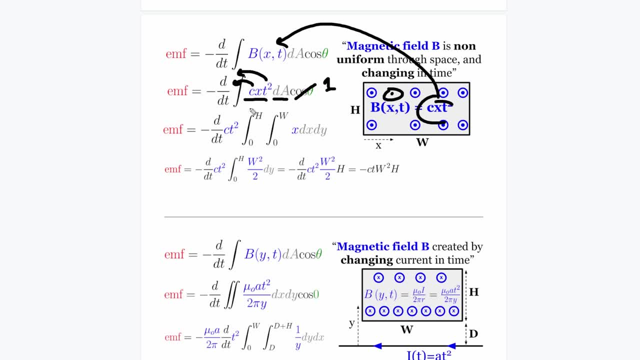 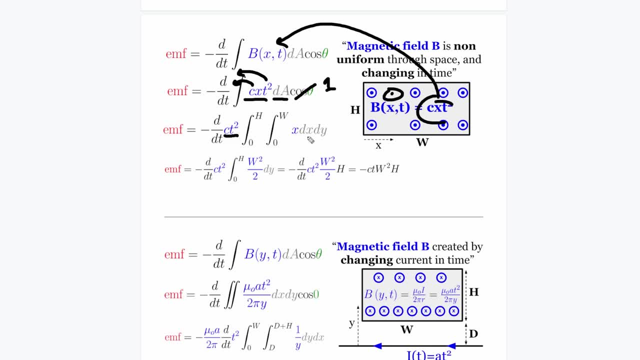 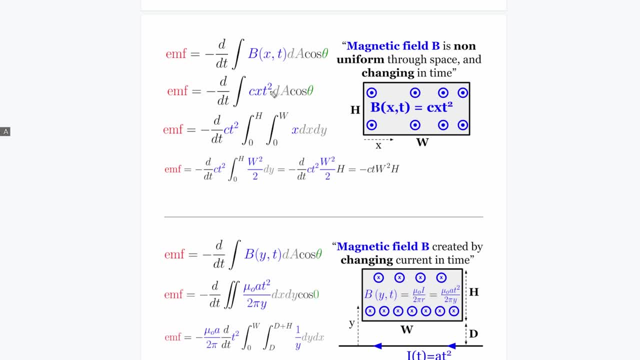 out of the derivative, but it can get out of the integral, And so you get this integral T or, sorry, X DA. You might be like what's DA? Well, it's a DX times a DY. So a little bit of height times a. 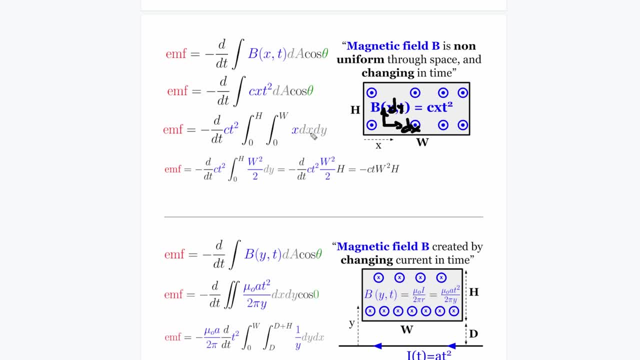 little bit of width, gives you a little bit of area, and infinitesimal area, But that's a double integral. How do I do that? Okay, That's okay. What you do is you say, Hey, I got nested integrals, I got my first integral here. Whatever comes out of this integral is going to be the thing that my 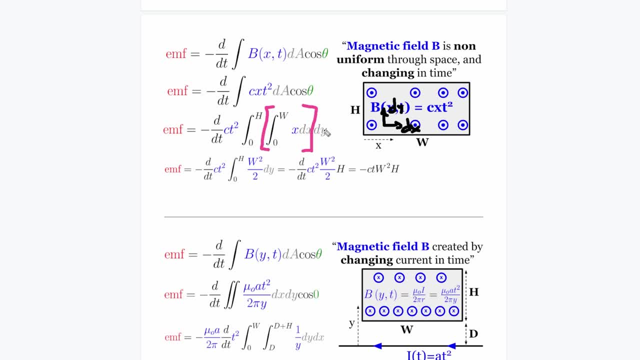 Y integral is going to integrate. So this is kind of nested in here and you can do them in either order, but I'm going to do the X one first, So my X integral happens first And it's like: Hey, what's the integral of X? Well, that's easy, It's X squared over two between zero and W, just gives. 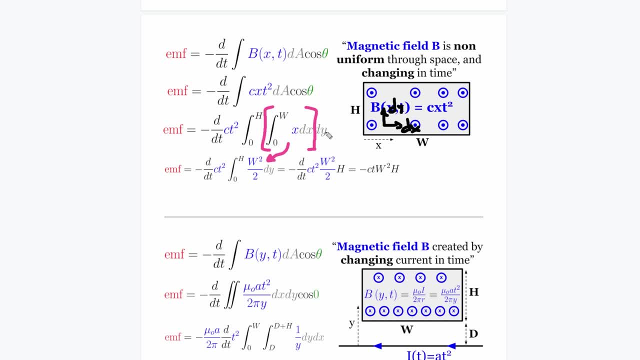 me W squared over two. And now, now, my Y integral is like: my turn, I'm going to integrate whatever you are. So the Y integral looks in here. It's like: Hey, anybody depend on Y? and W is like: no, I don't depend on Y, I'm the same W as high as you go. 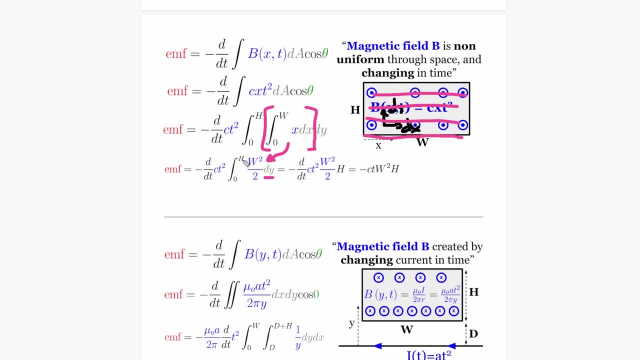 Same width. So these are all constants. It doesn't matter, You can take them out of the integral. Integral of DY is just Y. from zero to H just gives you an H. You get your W squared over two. You still had your CT squared weight. now, here And now your derivative acts your 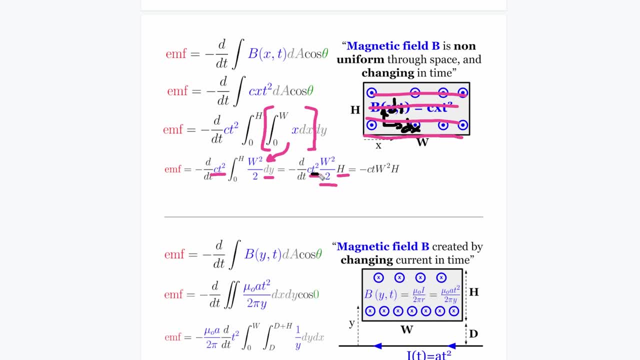 derivatives like: Hey, Hey, anybody depend on time. Well, the only thing that depends on time is T squared. So you get a two that'll cancel with this two, And you end up getting this as your EMF. You don't really care about the sign, Cause we're going to figure out that separately. 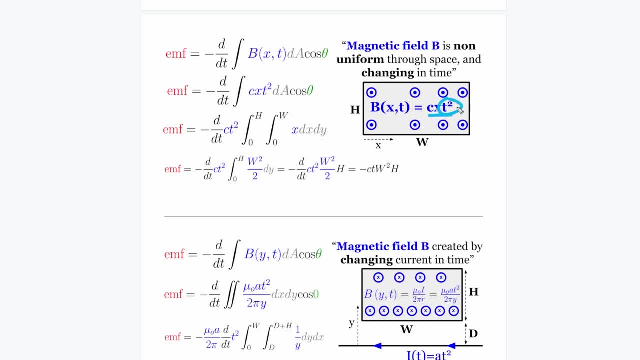 You ask yourself: does the flux increase or decrease? Well, it's increasing. as time increases. We're going to get more and more flux, So we'd be adding all this flux in here and our wires like no, no, no, no, no. I wanted to keep how much flux I had, So I'm gonna try to fight you with. 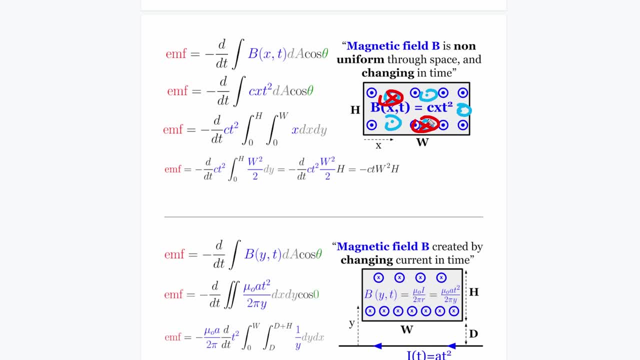 my own induced magnetic field. So we take our thumb pointed into the page and your fingers are going to be swirling clockwise. This is going to be the direction of the induced current created by this EMF volts. So that was that example. Uh, these might look hard but I do. 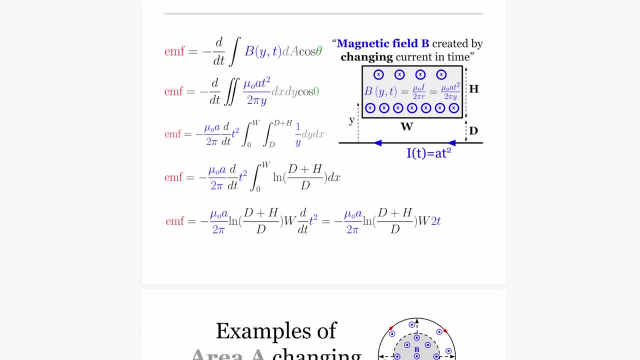 you gotta be ready for these, like an engineering physics class or an AP physics C. you're going to meet these. Here's a harder version of the one I just showed you. this time We actually get to discover what's creating the magnetic field. I told you it was an external 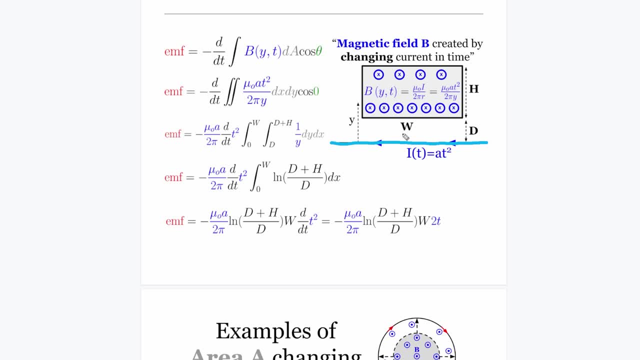 force or source. So here's a wire with a current. currents create magnetic field And this current is AT squared, So it's getting bigger over time And we can figure out which way the direction of the field points from this wire. You know, use your own right-hand rule, stick your thumb in. 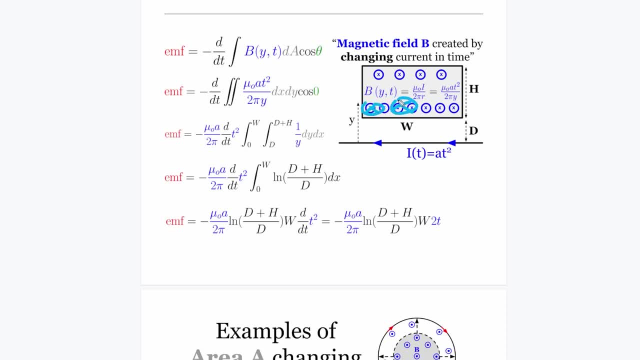 the direction of this current and your fingers will curl into the page up here. That's why I got X's. They're going into the page. If you see an X, an arrow, going into the page, what is all of this? What is mu not I over two power? Well, 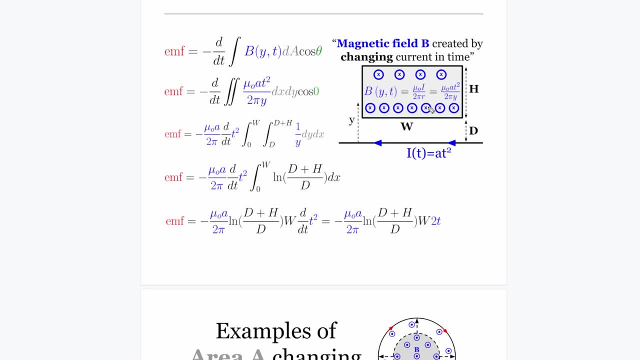 that's the formula for the magnetic field from an infinite straight wire. This comes up so often you should kind of just memorize it. You can get it from Ampere's law mu, not I over two pi R. So you take your I, whatever the I is creating that B, and we put it in there. That's why I have 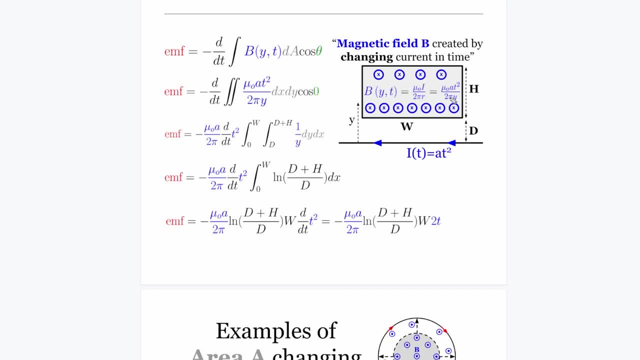 mu not AT squared, divided by two pi. Well, what is R? R is how far you are from the wire, So R is this Y direction, So I'm just going to call it Y. So this is my magnetic field, and it gets weaker as. 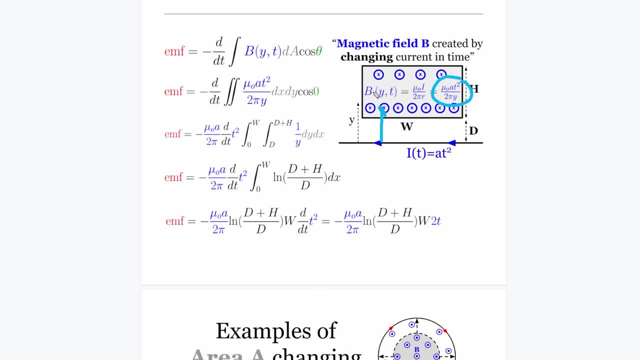 I go farther away, Like the bigger Y gets, the weaker B gets. So I have to do the integral version of this Faraday's law, because this area integral is like hey, hey, any of y'all depend on space, and the B is like, yeah, I do, I depend on Y. So I just, that's okay, Take this, put it in for B. 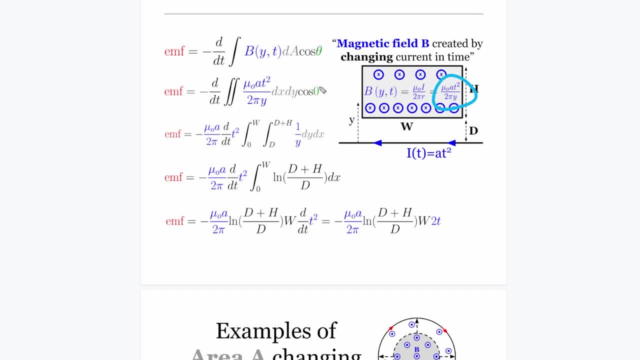 That's your B. I get DX DY. That's what my A is. My angle is still nice, Cosine zero. This gives me one. And then- sorry, let's clean this up- Who can sneak out of the integral? Anybody that doesn't. 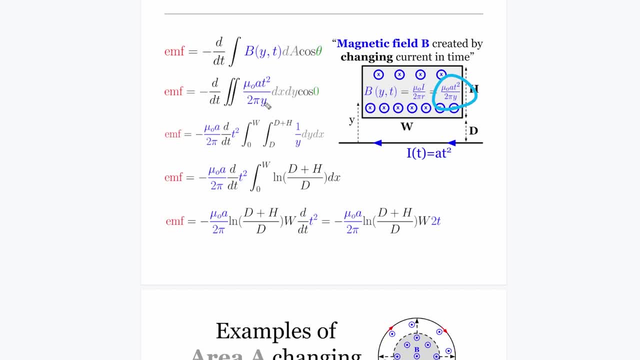 depend on X or Y. So that's everything, including the T squared, except for the one over the Y. That's the only thing that has to stay. Everything else gets smuggled out. In fact, everything else except the T squared gets. 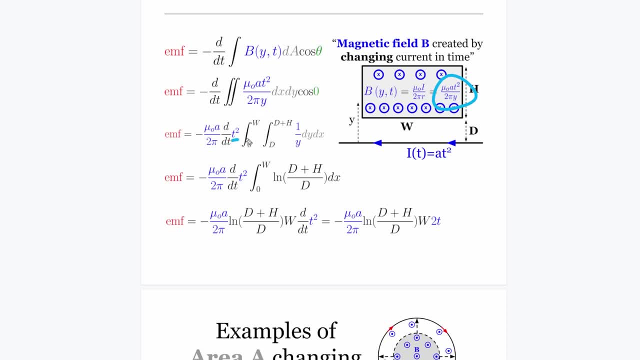 smuggled out all the way past the derivative. It's only the T squared that can't move past that derivative, because the derivative is checking for things that depend on time. Okay, So how do you do this? You do your integral first. We'll do the Y integral. 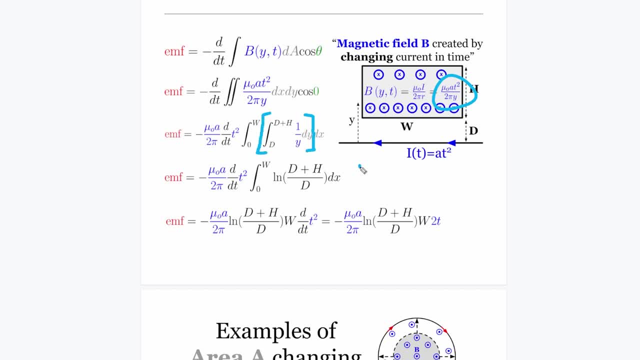 So I got one over Y DY. That's going to be log of Y. So what I'm going to get is like log of well, D plus H. You might be like: why is my limit D plus H? Because, look, the farthest I go is D. 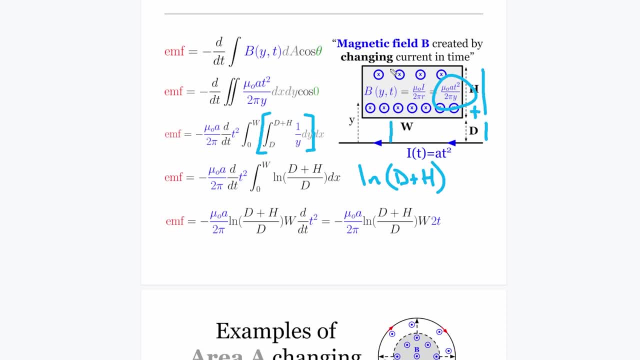 plus H And the closest I am in this hoop. we're worried about the area here. Remember it's this area. The furthest that area is in Y is D plus H. The closest it is is D, So I go from D. 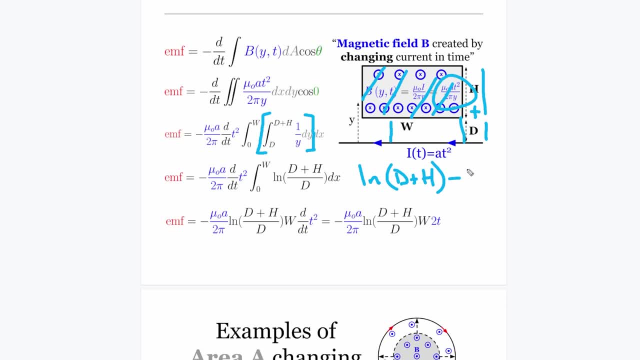 to D plus H, And so when I do that, evaluate that, I get log of the top limit minus log of the bottom limit. But the difference in logs is just the log of the ratio. So I can write this as this here: 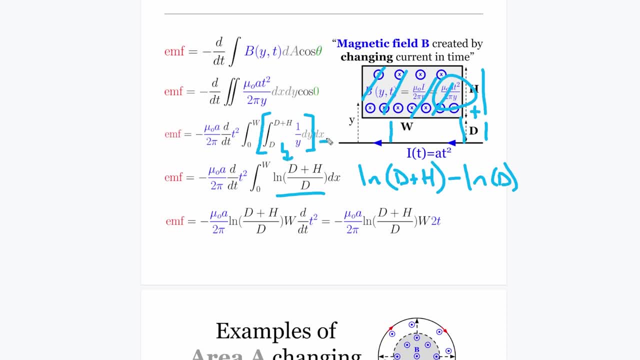 And now this comes down here, And now my X integral takes over. My X integral is like: my turn, I'm going to integrate anything that depends on X. And the X integral is like: oh man, there's nothing that depends on X here, So I can actually smuggle this whole. 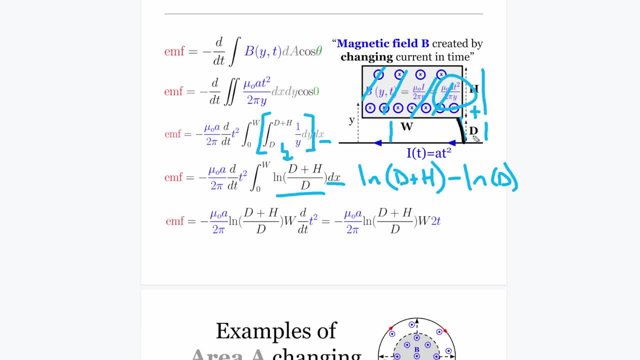 log out of this integral. Like this D doesn't depend on X, This H doesn't depend on X, Nothing there is X dependent. So integral of DX is just X. from zero to W just gives you a W, So you end up. 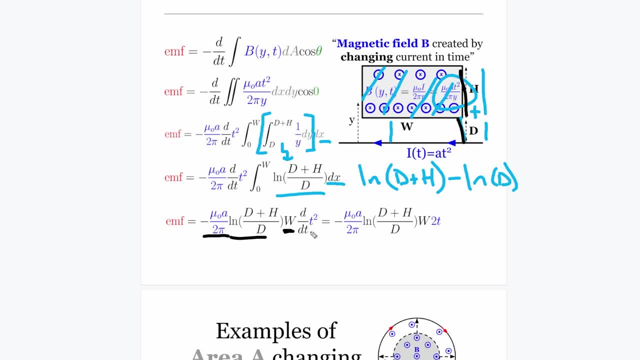 with this: log times, the W, all the stuff I smuggled out, And then the only thing that depends on time is T squared, So get the two T from that, So I get this right here And then again don't care about. 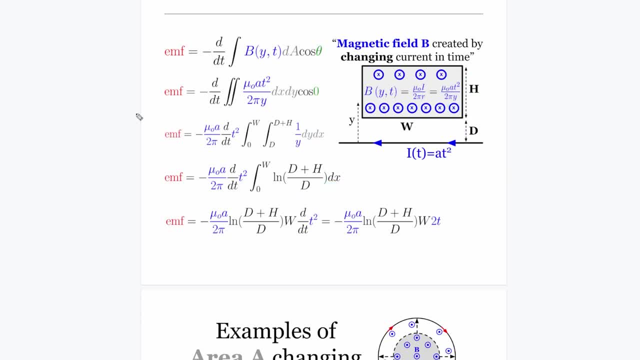 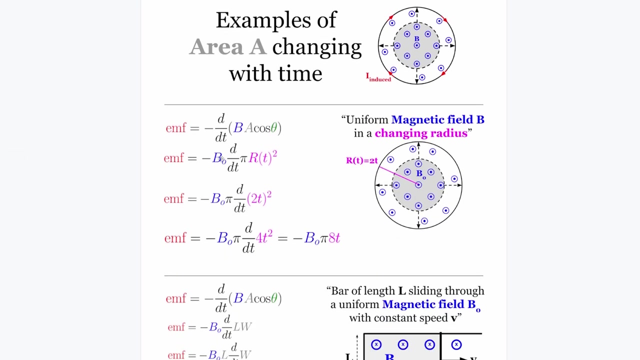 the sign, because we're going to figure that out separately. Does our flux increase or decrease here? Since the current's increasing, the magnetic field increases, we're getting more and more fields. We're getting more and more fields into the page And this copper hoop's going to be like: no, no, no, no, no, I don't want you. I'm going to try to delete you by creating my own. you know, I'm trying to cancel you by making my own magnetic field that comes out of the page. So put your thumb in the direction of this red induced magnetic field And you'll realize your induced current is going to be flowing that way. So that's about as hard as you get for the changing magnetic field examples. So you could change magnetic field. You could also change the area. What would that look like? So I'll say our magnetic field just stays the same forever, And it's usually the same. 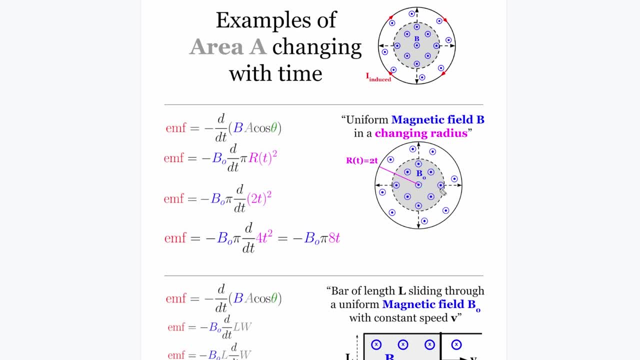 So it's uniform and it never even changes in time. It's just a constant b naught. So it's uniform. So we're not going to- we're definitely not going to have to do an integral here. We get to use the easy version of Faraday's law. So we take our b, whatever it is, we plug it into there. A is going to be pi r squared for a circle. Just you got to be careful. R is a function of time. now Our r is increasing in time two times t. So that's okay, We take that, we put that in here. pi times r squared: The r squared goes for r, but pi gets smuggled out, b gets smuggled out. Neither of these depend on time. So they don't get smuggled out. So we take our b, whatever it is, we plug it into there. A is going to be pi r squared for a circle. Just you got to be careful. R is a function of time. now Our r is. 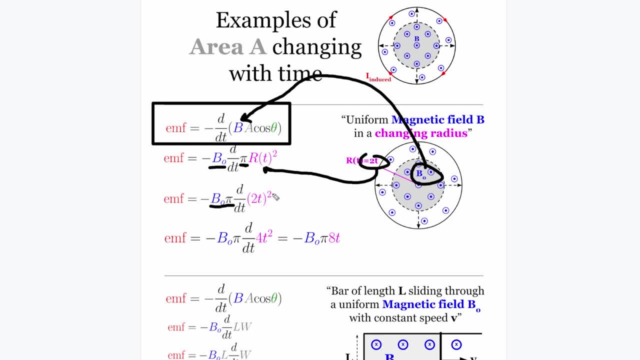 they get to get smuggled out the back door. for this derivative, 2t squared is going to be 4 times t squared. The derivative of that is just 8t times b0 times pi. Which way does the current flow? Well, did flux increase or decrease here? Flux increased. We're gaining all these extra arrows. 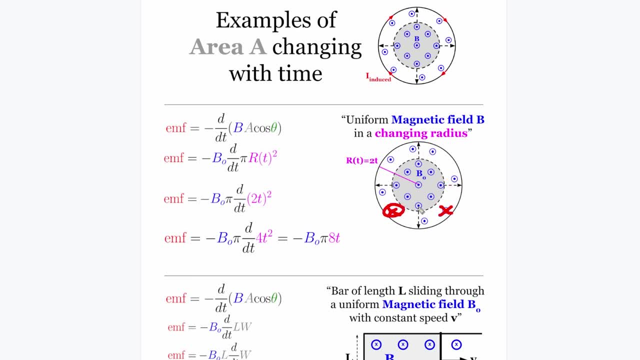 out of the page. So our wire is going to be like: hey, I want to get rid of you, So I'm going to make my own induced field that goes into the page. Stick your thumb into the page and you realize your induced current would go that way. So that was one example. Here's another example. you see a. 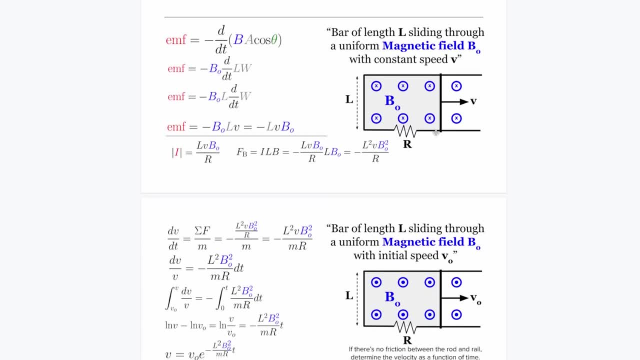 lot If you got a rod sliding on a like hoop right here. this, like you know, this rectangular hoop and a rod slides on it and there's an external magnetic field. So in other words, this rod looks like here and it's going to be over here at some later point And it's like over here And 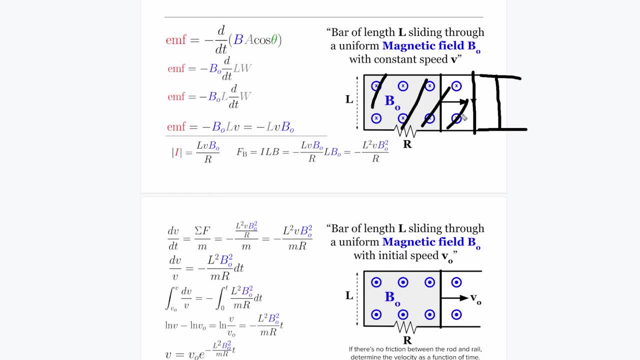 this keeps going on forever. You're increasing your area. This is an example of increasing area. So how do we do this? Well, same old Faraday's law and the B field's uniform B is the same Everywhere, to the right and vertically, So we can use the easy version without the integral. 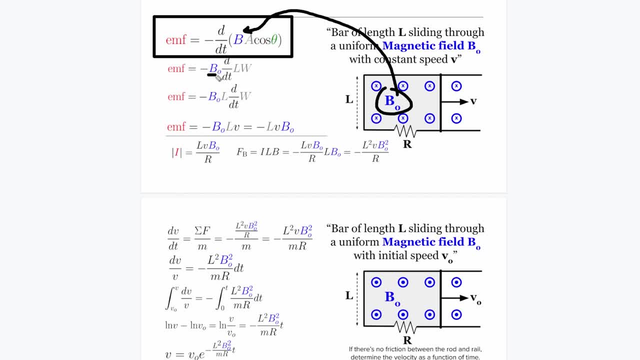 So we take our B, we take that, plug it in there And that's a constant. We can smuggle it out the back door. that derivative. We take our area. That's going to be length times width. You might be like I don't know the width, That's okay, Just write it as length times width. The angle's. 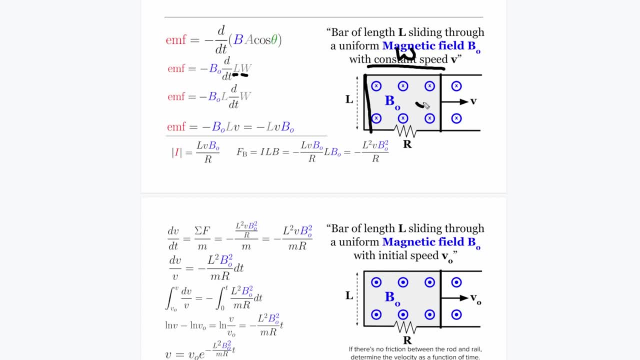 still nice Angle comes out of the page. Oh well, let's define the area as like into it. We're going to get rid of the sign anyway, It honestly doesn't really matter. But anyways, the angle gives you a cosine of either zero or 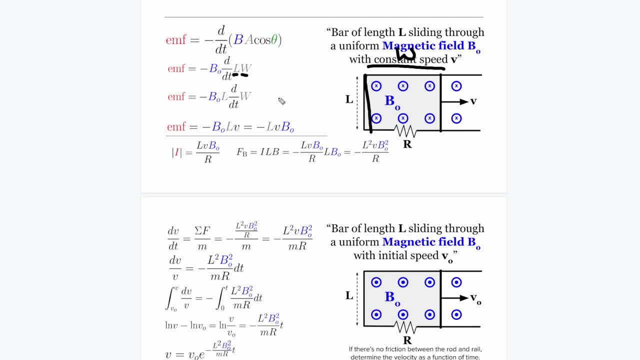 180.. You either get one or negative one here, but we don't care, because we're going to get rid of the sign in a minute, All right. So this derivative is like: Hey, who in here is changing in time And. 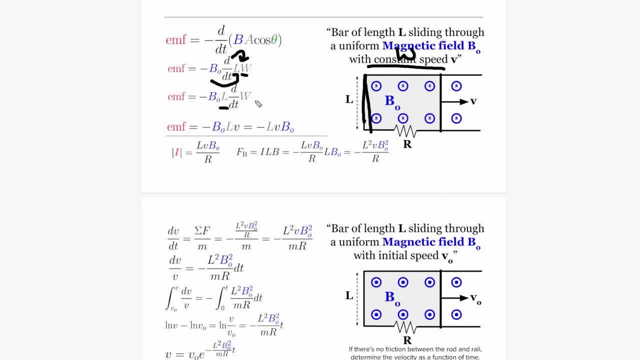 the length is like, not me, So okay, You can sneak out the back door. How about W? Yeah, W changes. Look, the width of this rectangle gets bigger and bigger in time. And you might be like: well, I don't know what the derivative of W is, but you do If the speed of this rod is V. 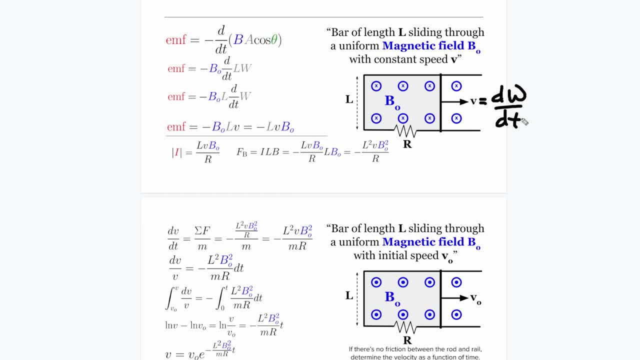 V is how fast you're changing the width in time. If this is moving to the right at three meters a second, you're gaining Three meters of width a second. So DWDT is V, So you just get. BLV is the EMF. This is important. 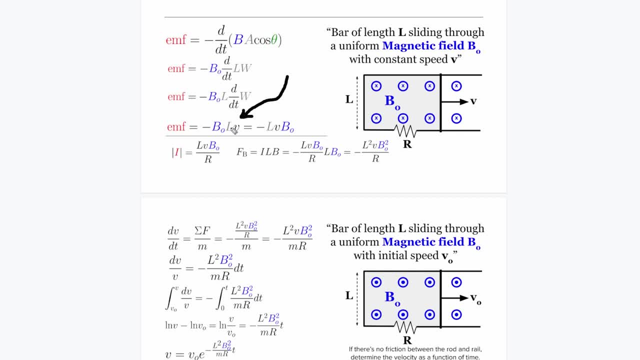 Like this result comes up so often, You should just memorize it. But I like memorizing like this. I rearranged the letters. I call it LVB because this looks like Las Vegas Boulevard And if you've been to Las Vegas Boulevard, there's a lot of volts. on Las Vegas Boulevard There's lots of. 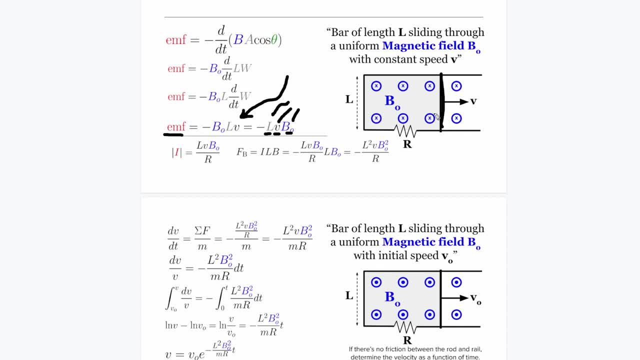 lights and stuff. So LVB equals the EMF from a rod moving through a field. So that's cool. You could get that If you knew the resistance. take LVB, The volts over R, that gives you the current. Which way would the current flow? Well, we're. 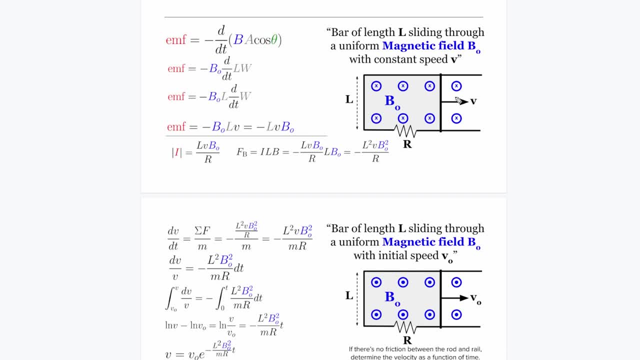 increasing flux. Our flux is increasing. We're getting you know this rod will be over here And it's like dang. now our area is including all of these as well, So our hoop's going to be like: no, no, no, no, no, I'm going to get rid of you. I'm gonna try to cancel you by making a. 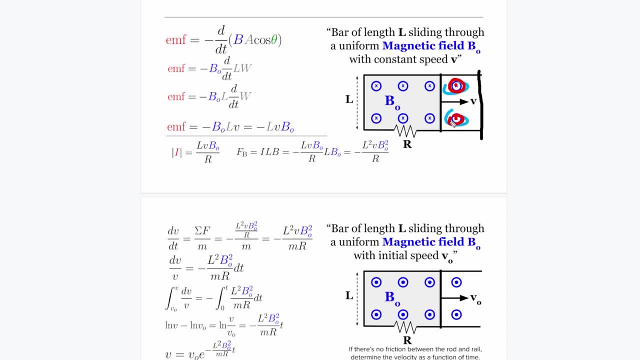 field the other way. So since we increased flux, I'm going to put my thumb in this direction out of the page And I get that my current's going to be flowing in this direction. It'll be this big And if I got a current flowing in a magnetic field, I'm going to have a 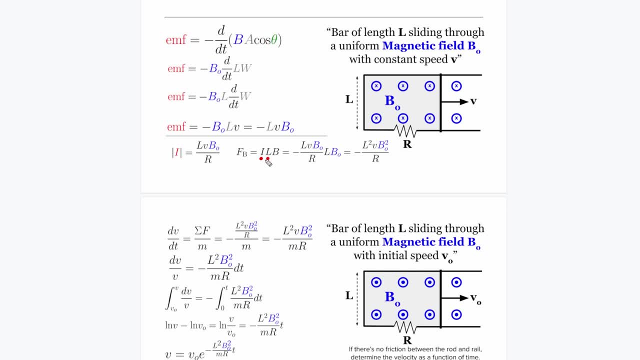 force. The force is ILB filled, And so I take my I. this is my I. I put it right there. I take my length. Well, this was my length of the rod, I put it right there. I take my magnetic field. 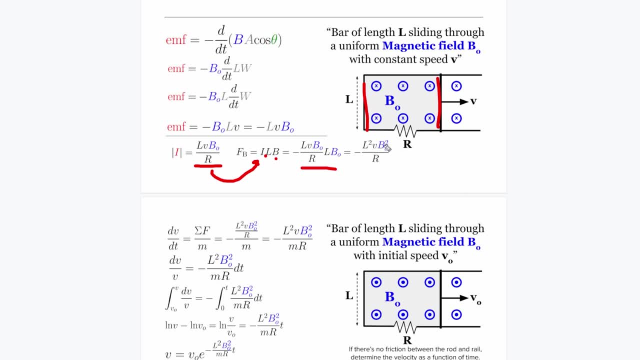 I multiply that all out and I get L squared V, B squared over R. That's the magnetic force. Which way does it point? It points backward. Magnetic force is a hater force. It's going to oppose. whatever you do, You try to pull a rod to the right, magnetic force to the left, So you 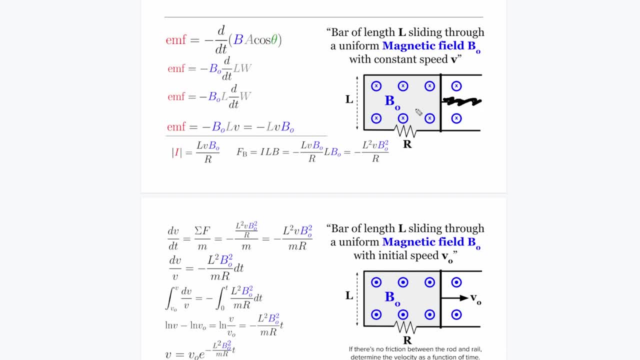 might be like: well, what if I, what if I push the rod to the left? And what if I get the rod going this way? Well now, because flux decreases, everything switches and your magnetic force this time is going to be to the right. It's like no, I'm going to. 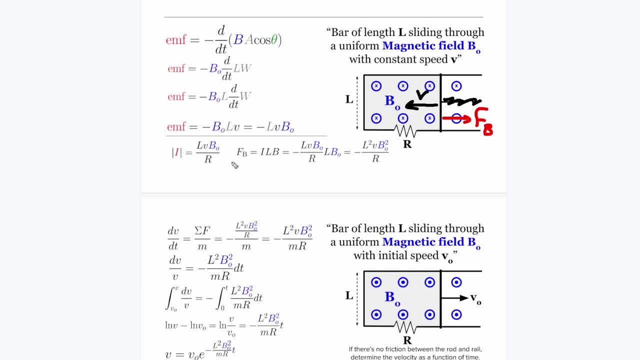 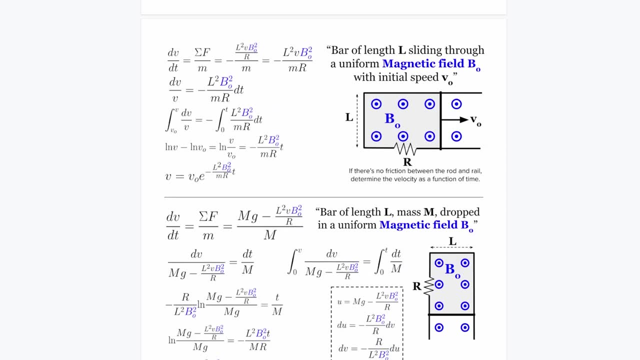 oppose. whatever you do, It's like a damn. you change the flux, magnetic force is going to oppose you. So that's a hater force always against what you do. So that's a common version, LVB. So it comes up a lot. Uh, in fact you can think of complicated versions here. This might look. 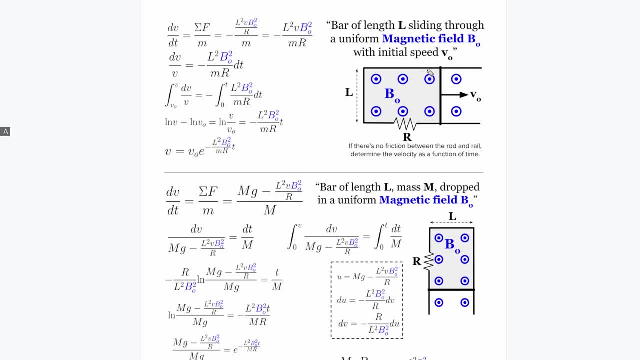 overly complicated, but I swear you're gonna have to do this If you're in an engineering class or AP got to know how to do this. If the rod slides with an initial speed, V naught no friction between the rod and the rails. What's the velocity as a function of time? 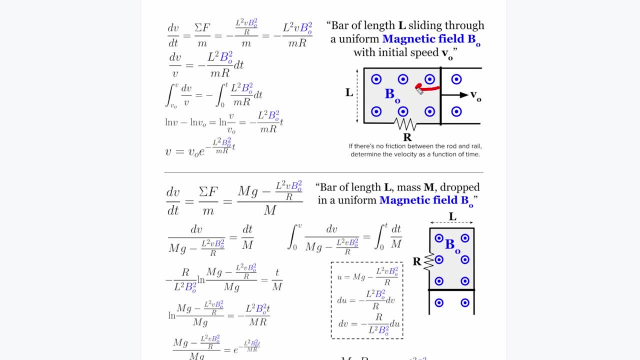 So, first of all, this is going to slow down. It's going to slow down because, remember this, this magnetic force is a hater force opposing you, So it's going to slow you down. So, what is the velocity as a function of time? Well, you got to do Newton's second law, You do. 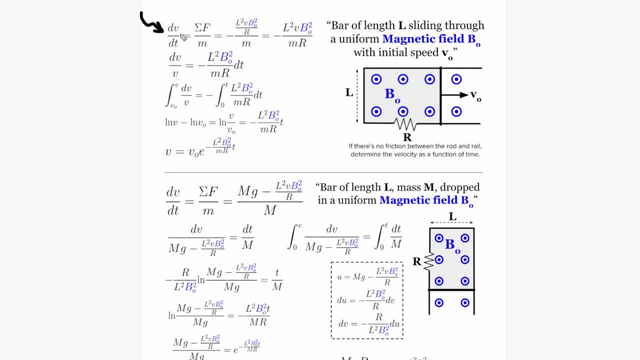 a is net force over M and we're writing a as DVDT because you want a differential equation. What's my force? We just found that in the previous problem the forces L squared V, B naught squared over R with a negative. The negative is important. 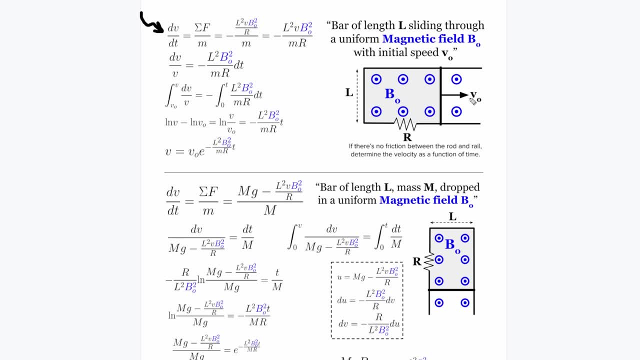 It's saying it's opposite direction of the V. So that's what the force goes: opposite direction of the V. I divide by M. Uh, I can like combine that stuff together. At this point I have to do the separate, integrate, celebrate. I got my V's and my T's. Those are my only variables, So I got to. 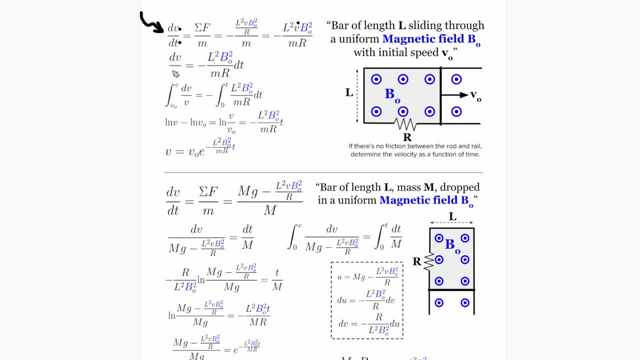 separate the V's from the T's. first step separate. So I put my V over here, I divide by V, I move my T over there, I get this over here. So I've separated. Now I integrate step two, So I. 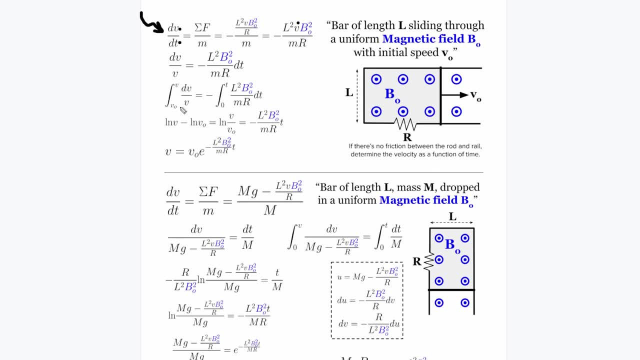 integrate both sides. integral of DV over V, That's just log V between V naught and V would be log of V minus log of V naught. I integrate this side and this integral is like: Hey, anybody in here depend on time And this L is like no ma'am, B's like no ma'am, no ma'am, no ma'am, I got no time. 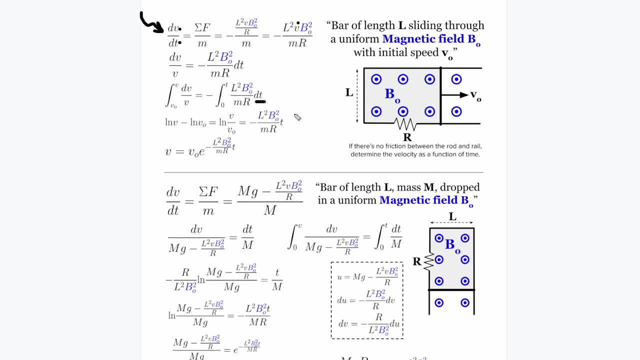 dependent. So these can all wait out front and I get integral of DT. Well, that's just T between zero and T. That just gives me T. So I get this right here and I could log. I could write the difference of logs as the log of a ratio. How do I solve this for V? I'm trying to solve for V. 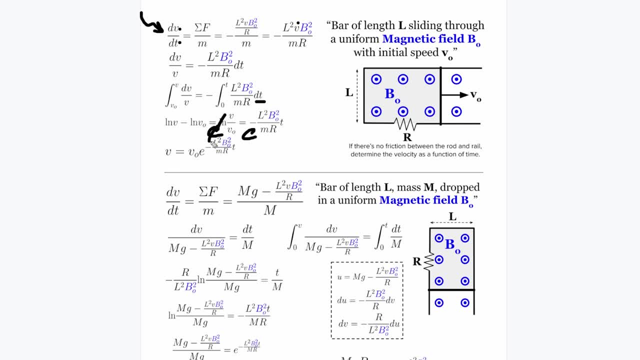 This here is my V that I'm solving, for We'll take E to the both sides. E cancels log. I get V naught, E to this mess, So I just multiply by V naught and I get this right here. So this is my velocity. 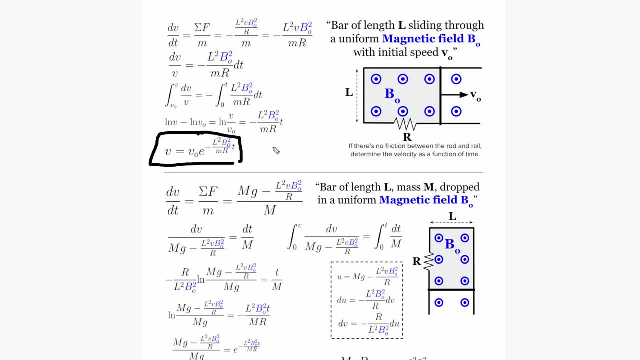 as a function of time. Notice it's V times E to the negative. So it's going to look like this: as time increases, I start with some speed and it dies off like an exponential in time. So that's what that looks like. Okay, That's honestly. this is the easy version of this problem. The harder 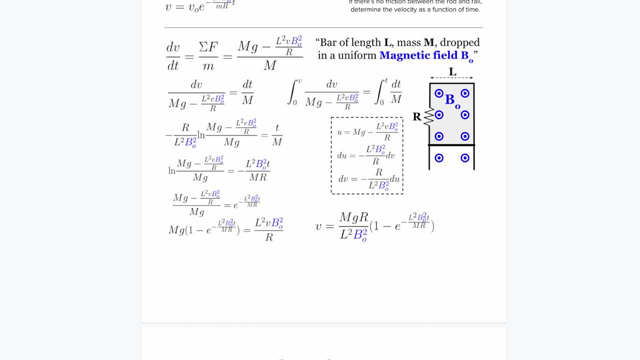 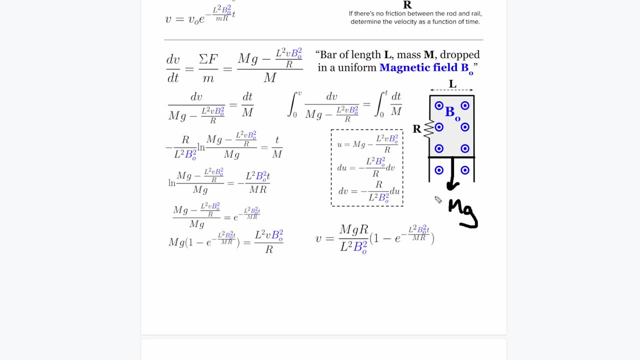 versions down here and you need to know how to do this one too. Like this is expected that you know how to do this. Let's say I took the rod and this time I let it fall in gravity. So this time there's a force of gravity. this way This is like downward. So I got my magnetic force, my magnetic. 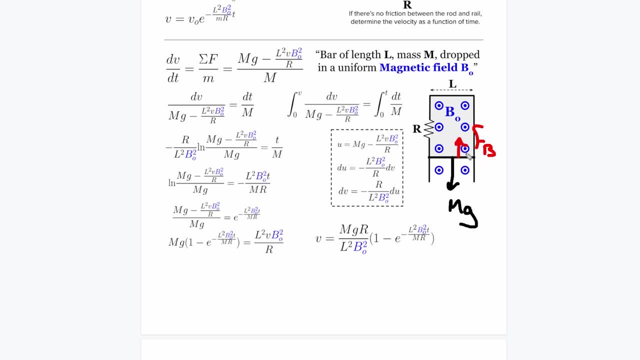 force, the hater force, is going to be pointing up. It's like: Hey, I don't want you to change my flux. So these two are opposing each other. So it's the same situation. Let's say we wanted to find the magnet or the velocity as a function of time. here We do Newton's second law: accelerations. 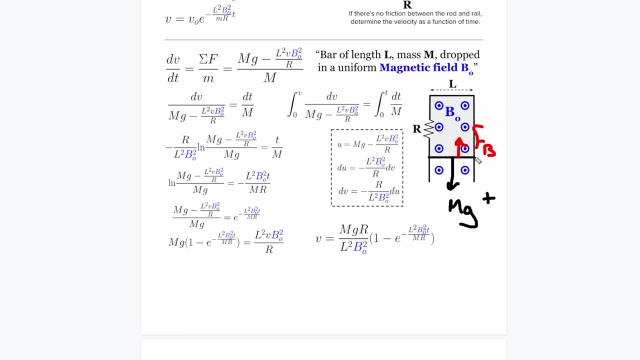 force per mass. So I have MG down. I'm going to call this direction positive, because if you call the direction of motion positive it just makes it easier. So MG is down minus. I got this magnetic force here over M. So again I have to separate, integrate, celebrate here. So 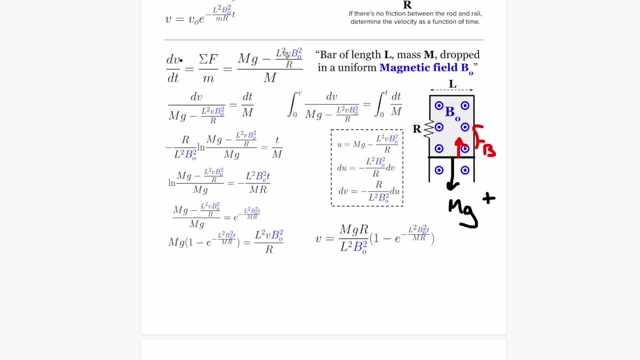 V and T are my variables, So you might try to separate this MG from all of these, but you can't do. you got to treat this like a family. This family moves together. So I take this whole thing and I divide over here- So I'd have DV over this whole mess- And then I move DT to the other side. 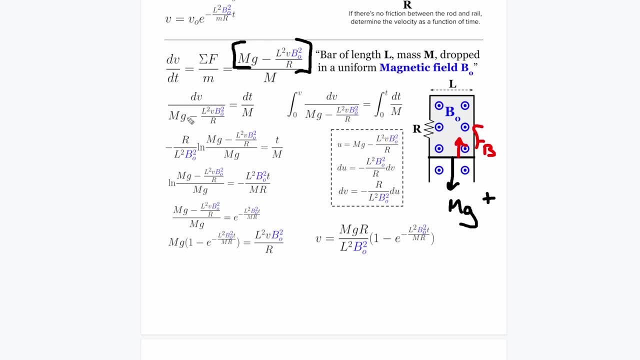 get DT over M. All right, They're separated. Now I integrate. Now you have some. you know you could divide by M's if you want, but like this whole something minus something's got to move over here. You're never going to be able to separate it, And now I can integrate both sides. 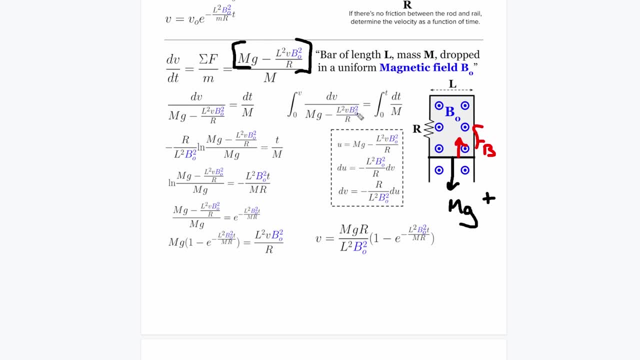 This time you're like: dang this integral is hard DV over all this mess. I got my V here. What do I do? Well, you use substitution. So call this whole bottom thing U. So I'm calling that whole thing U DU. that would then be, you know it. 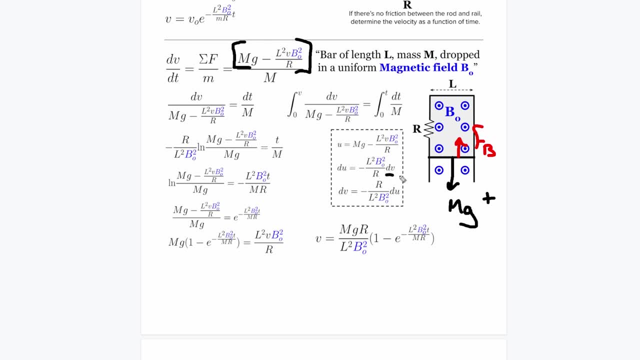 annihilates that I get L squared. B naught squared over R times DV. Solve for my DV. I'd get DV as this negative mass times DU. So what I'd get is that you know, up here I'd have R over L squared. 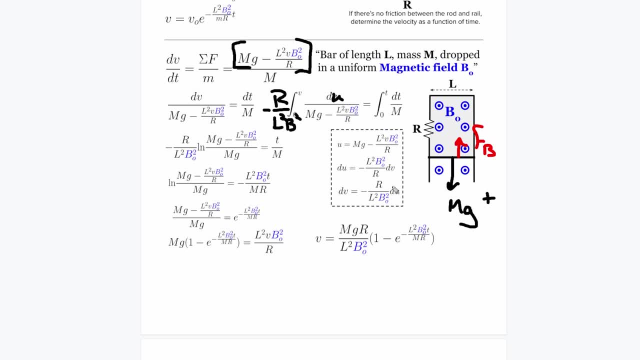 B squared negative. This would be DU if I subbed in for DV And then all this down here would just be U, So I'd have integral DU over U. but integral DU over U is just the log, So I do the same thing. 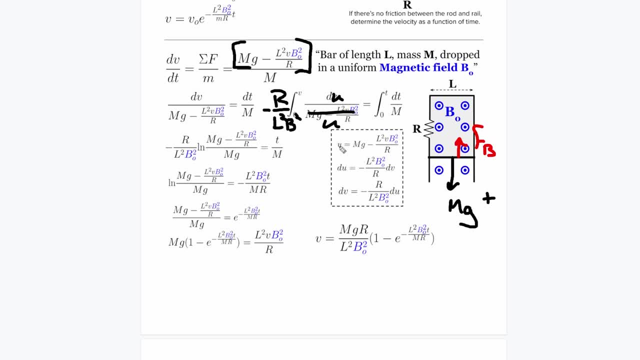 Log of the. you know difference of logs, but I could write that as the log of the ratio. you know, log of the ratio. and be careful, The zero limit here, the zero limit, doesn't give you zero. You plug that zero limit in and you get MG. It's not zero. So be careful, You get a difference. 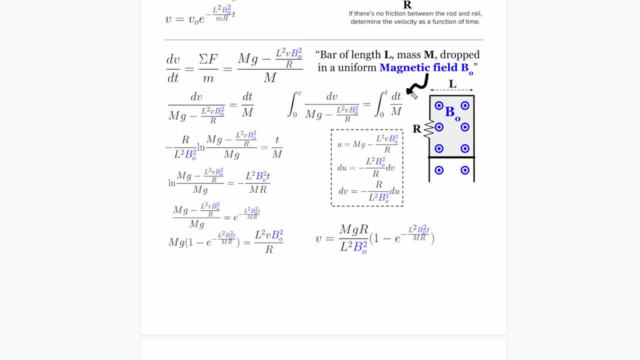 of logs and you get the log of the ratio And then over here it's easy. This integral is easy. Integral DT is just T over M. So you get this whole mess here. Uh, you know, multiply both sides, you divide both sides. by that You get this here. take E to the both sides. 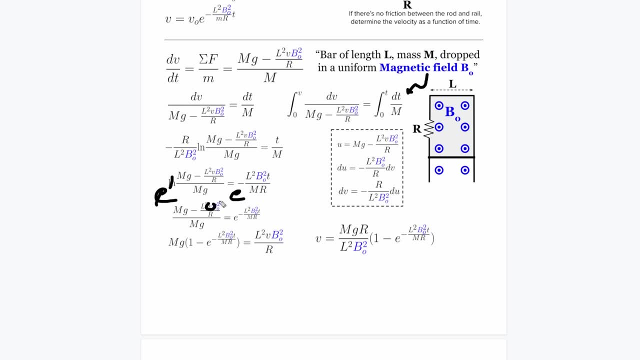 log gets canceled And then it's just a bunch of algebra that I don't want to bore you with. You solve for this V. This is what you're trying to solve for This V is a function of time, So you solve for that V and you finally get this over here. What does this look like? Well, 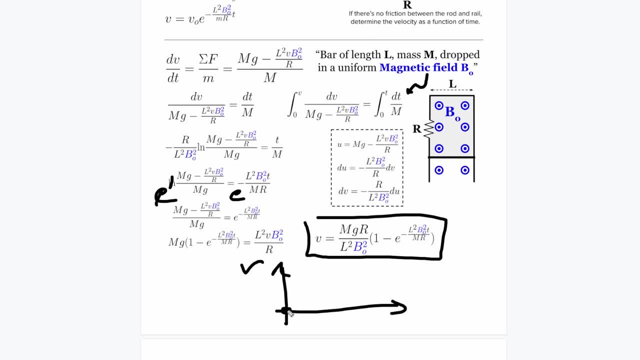 if you graph this this time we dropped it. it started at rest and it looks like that And it gets to some terminal velocity And you can find that by just being like: well, what if I plugged in? T equals infinity. I'll wait a long time. 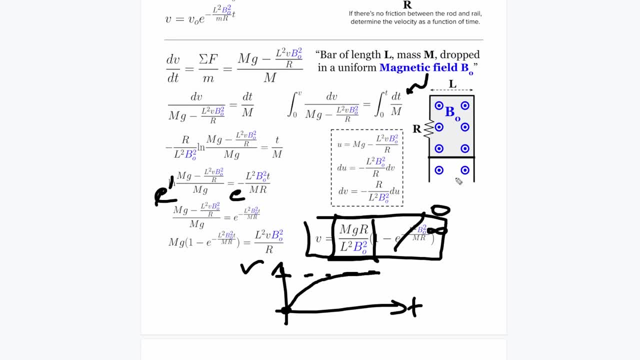 Leave the negative infinity zero. So this here would be your terminal velocity. Eventually you'd get to some terminal velocity where the magnetic force upward and the gravitational force downward would just cancel And it would just move at that speed right there. Okay, That's about as hard of a 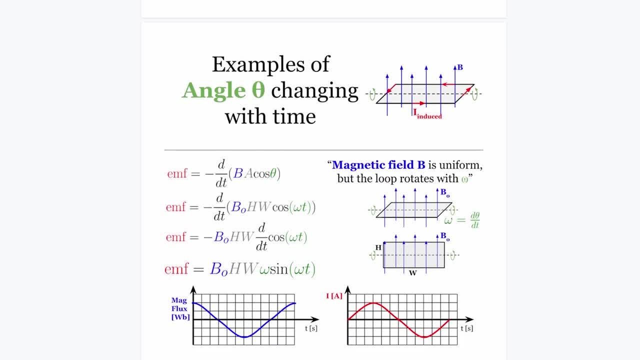 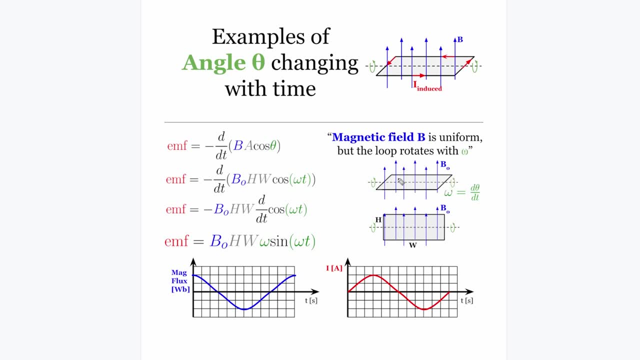 problem, as you can get where the area changes. There's only one more problem I want to show you: What if the what if the angle changed? How would you even do this? Well, you'd take like a rectangle, You just start rotating it in a magnetic field so that right here it's catching a lot of. 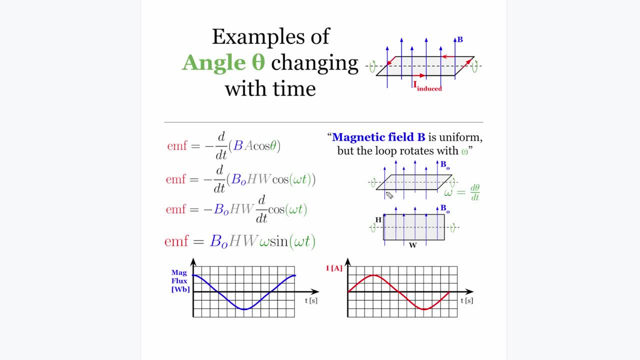 flux And now it's in this orientation of catching no flux And it just keeps rotating. It's changing its angle. This is actually how most power plants work. It's actually easier to do this: You burn something that spins something and you get a lot of volts out because you've got some 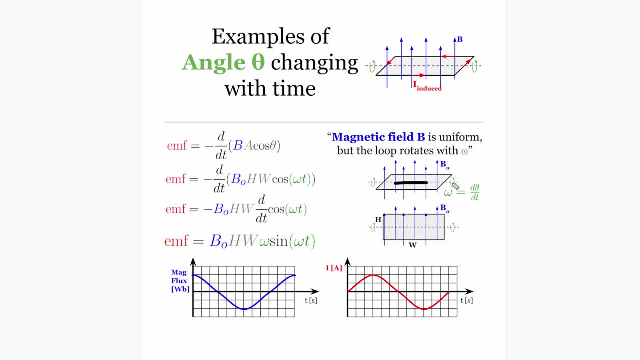 magnetic field here and you're using Faraday's law. but look at this: magnetic field uniform, doesn't depend on space. So we could use the easy version of Faraday's law. I take that, I take whatever my magnetic field is. B naught, I put it in there. That's why I got this area height times. 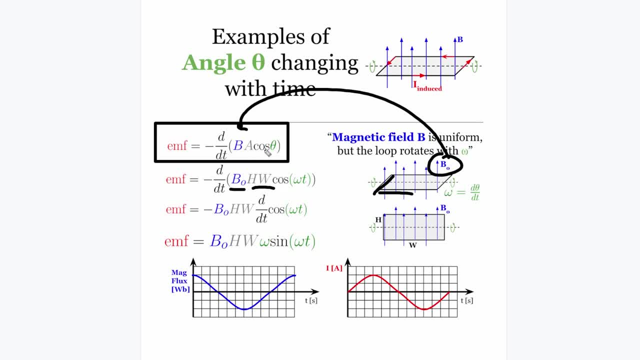 width easy. This time, cosine theta is not our friend. This time, cosine theta is the complicated equation. We're just going to use the. What if we wanted to write this? Well, if you remember, you know Omega, the angular rate of. 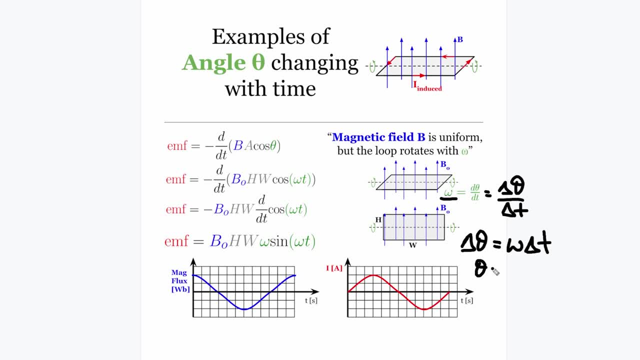 spin angular velocity is d, theta dt. or you could just think about it like: let's say you're spinning at a constant rate, It's how much theta you go through per time. So if we wanted how much put it in for theta, I'm gonna call that omega t. So I get this whole thing. And now we got our. 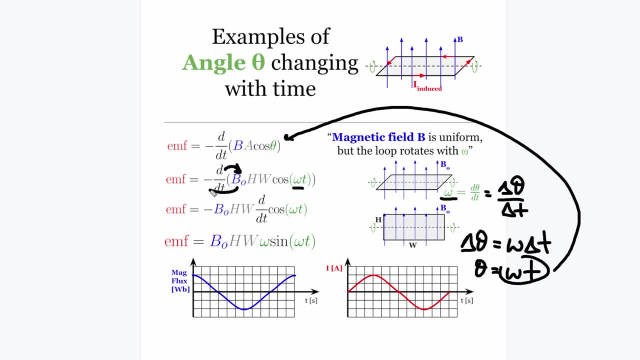 derivative, checking everyone out, like hey, you depend on time. No, sir, you can sneak out the back door, H and W sneak out the back door. This is the only thing that depends on time. So we take a derivative of this cosine omega t, But the derivative of cosine is sine. But we got to do. 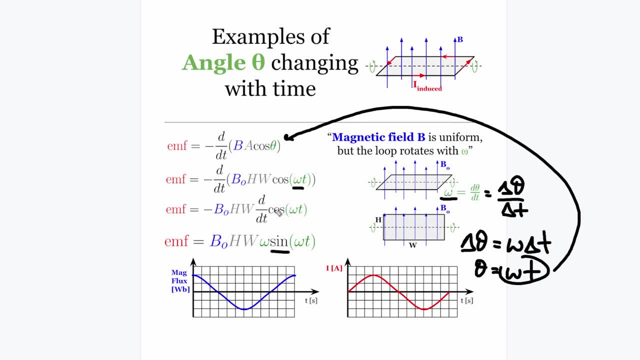 the chain rule here. In fact it's negative sine. That's why the negative got canceled. But we don't care about the negative. anyway. You got to take a chain rule. So derivative is cosine sine. but then you got to take a derivative of the inside with respect to time. that gives you an omega out. 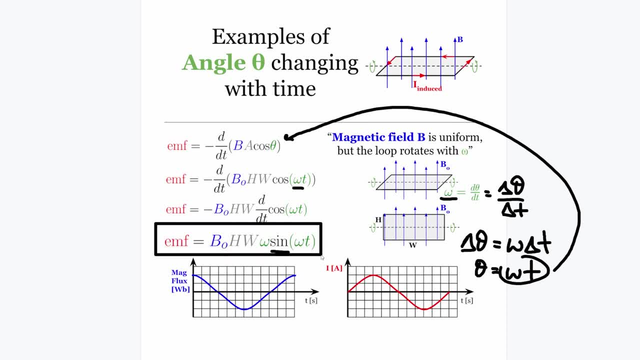 here, So you get this right here. this is going to be our EMF: how many volts we get And, if you notice, it depends on omega, like the faster you spin this thing, the more volts you're going to get, And it's going to be varying in time. So this EMF which, if divided by resistance, gives you the 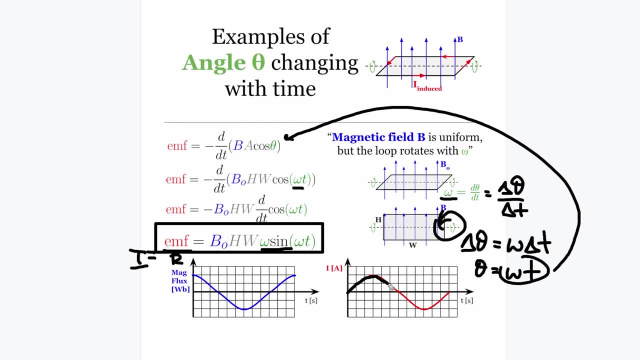 current. it's going to look like sine, So it looks like this, because our resistance is just a constant, you know. so whatever EMF looks like functionally is what I looks like, So it looks like a sine. But our look at this was our flux. ba cosine, theta is our flux, So it's going to be.